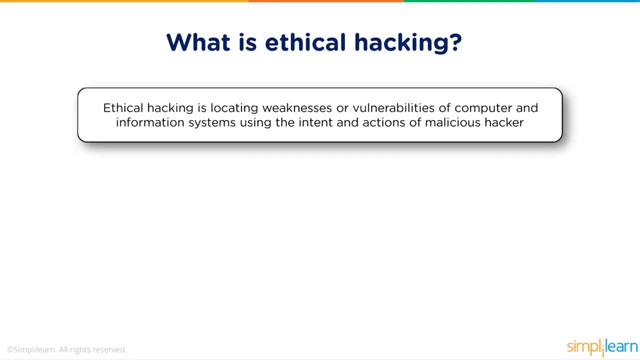 activity. I cannot in good faith hack somebody and then tell them: you know what? I just wanted to help you out and here are your vulnerabilities and this is the way you can prevent them. I first need the authorization from the other party, and only then can I perform an ethical hack. So in this example, 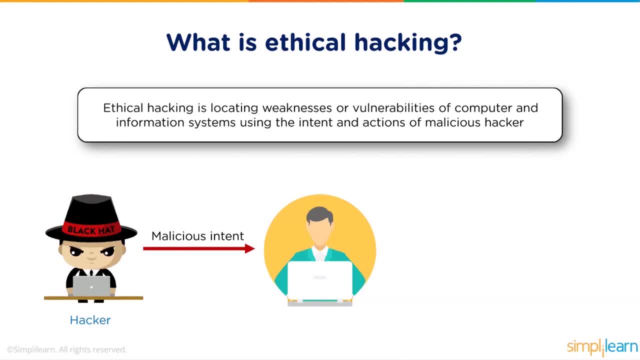 hacker attacks an individual with malicious intent and makes misuse of whatever information they have gotten. They steal the data, they maybe fry the operating system hardware, destroy it and thus they leave the victim without a device. With authorization, an ethical hacker can also attack the same individual, minus the destruction of course, and the intent is good. so they are willingly. 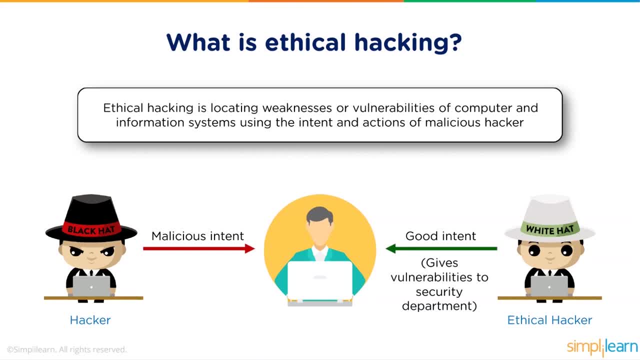 finding out the vulnerabilities and helping the victim plug them out so that they wouldn't be a victim of a malicious attack. Now, here the first thing is authorization from the victim and the second thing is the good intent, where we do not misuse those vulnerabilities and we report them. 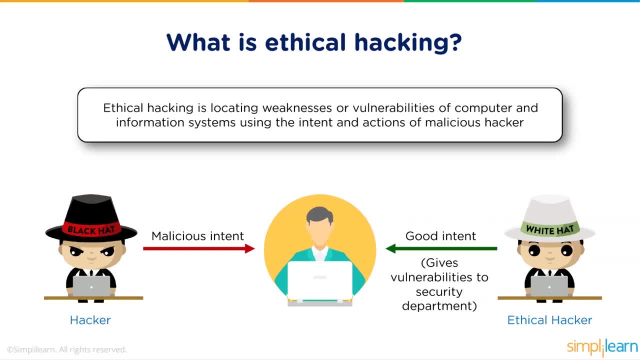 back to the victim. We report them back to the client and help them patch those vulnerabilities. That's the main difference between a white hat and a black hat, So security experts are normally termed as white hat hackers. Malicious hackers are termed as black hats. Now, the responsibilities of an ethical 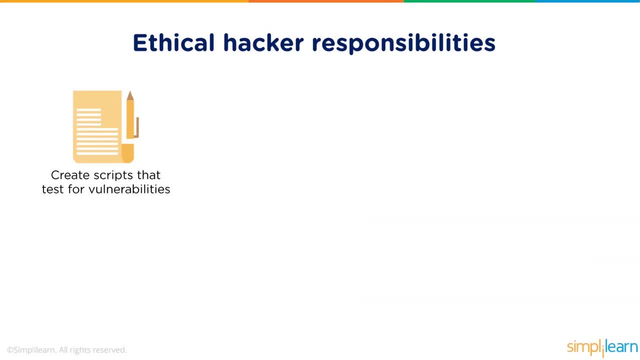 hacker are multifold. First and foremost, you have to create scripts, test for vulnerabilities. First. you have to identify those in the first place. So there's a vulnerability assessment identifying those vulnerabilities, and then you're going to test them to see the validity and the 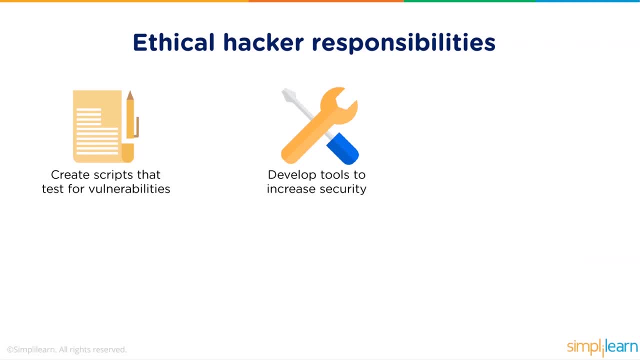 complexity of the vulnerabilities, So you have to identify those in the first place. So there's a vulnerability assessment identifying those vulnerabilities, and then you're going to test them to see the validity and the complexity of those vulnerabilities. So one of your responsibilities would be to develop. 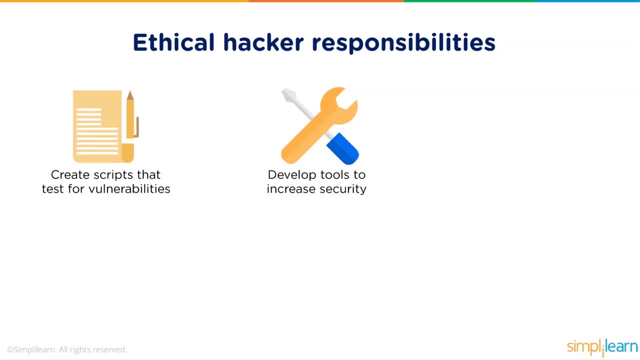 tools to increase security as well or to configure security in such a way that it would be difficult to breach Performing risk assessment. Now, what is a risk? Risk is a threat that is posed to an organization by a possibility of getting hacked. So let's say, I, as an ethical hacker, run a 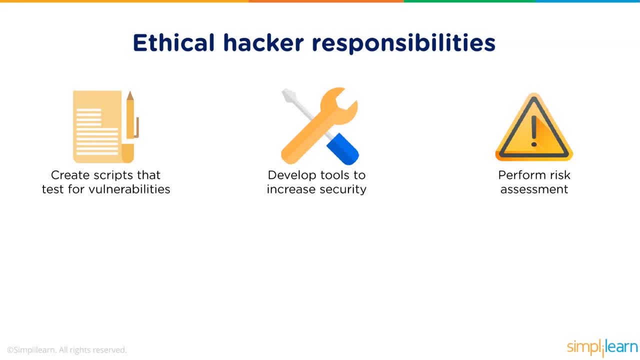 vulnerability scanner on a particular client. I identify 10 different vulnerabilities Within those 10 vulnerabilities. I do a risk assessment to identify those vulnerabilities and then I do a risk assessment to identify which vulnerability is critical, would have the most impact on the client and what would be the repercussions if those vulnerabilities actually get exploited. So I'm 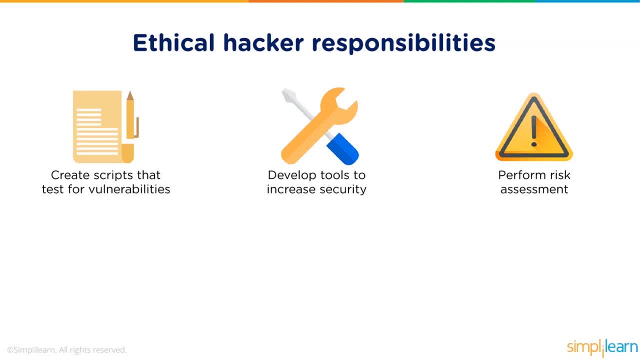 trying to find out in risk assessment that if the client gets hacked with the vulnerabilities identified, what is the loss they would be facing once they get hacked? And the loss could not only be loss of data, it could be financial losses, it could be loss of reputation, penalties they have. 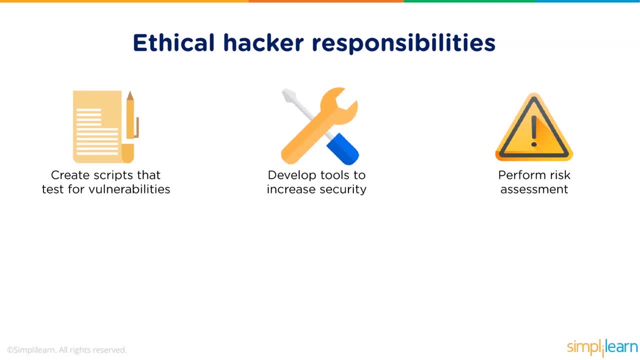 to pay to the client for breaches or penalties that they may have to pay for. pay the governments in case of breaches that happened that couldn't be controlled. Another responsibility of the ethical hacker is to set up policies in such a way that it becomes difficult for hackers to get access to devices or to protected data, And finally, train the staff for 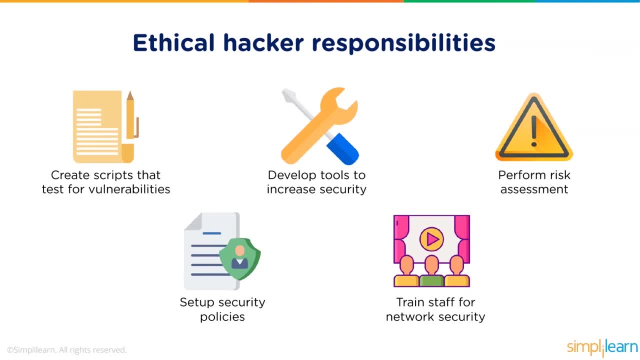 network security. So we've got a lot of employees in an organization. we need to train the staff of what is allowed and what is not allowed, how to keep themselves secure, so that they don't get compromised, thus becoming a vulnerability themselves to the network security. So I'm 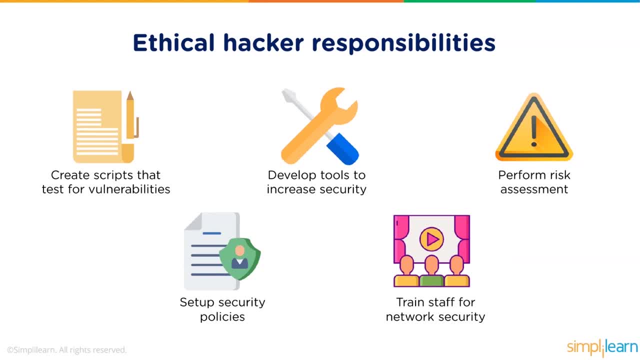 going to talk a little bit about the policies of the organization. The policies that we have talked about are administrative policies to govern the employees of the organization, For example, password policies. Most of the organizations will have a tough password policy where they say you: 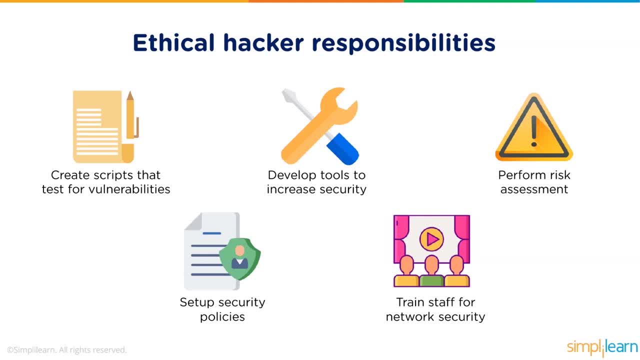 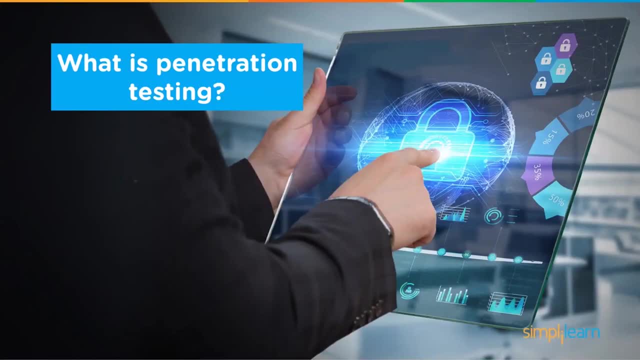 have to create a password that meets a certain level of complexity before that can be accepted. And till you create that password, you're not allowed to log in or you're not allowed to register. So let's move on to understand what is penetration testing. Now for penetration testing, there is a 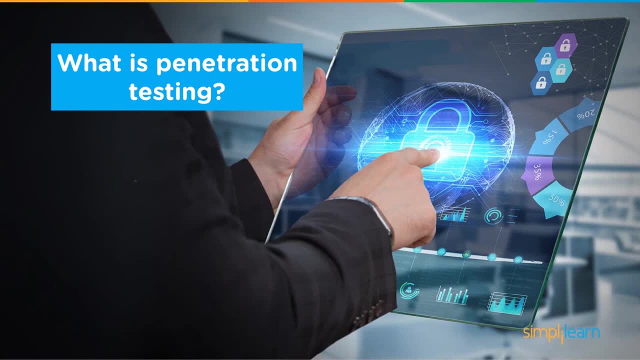 phase, called vulnerability assessment, that happens before this. Vulnerability assessment is a phase that happens before the validation of a system. Vulnerability assessment is nothing but running a scanning tool to identify a list of potential flaws or vulnerabilities within the organization. Once you have identified the list of those vulnerabilities, you would then move on to 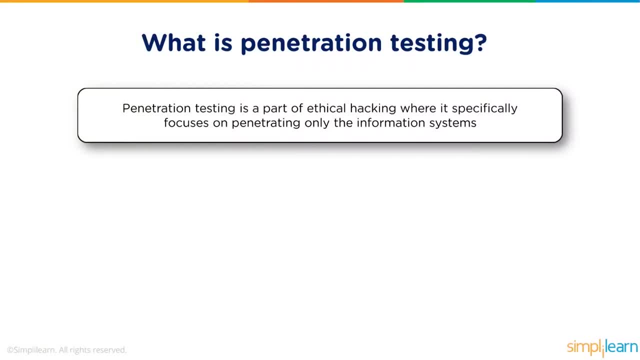 penetration test. This is the part of ethical hacking where it specifically focuses on penetration only of the information systems. So you have identified that flaw. Maybe it could be a database with a SQL injection, or it could be a buffer overrun flaw, or it could be a simple password. 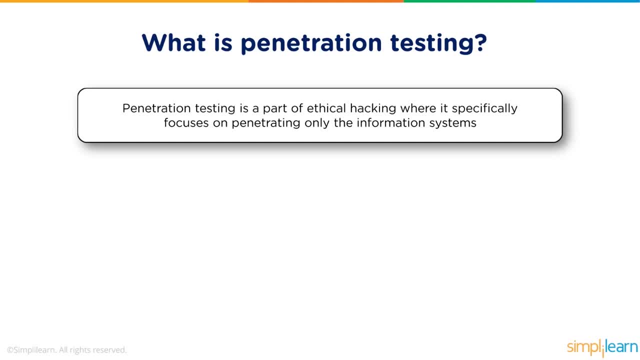 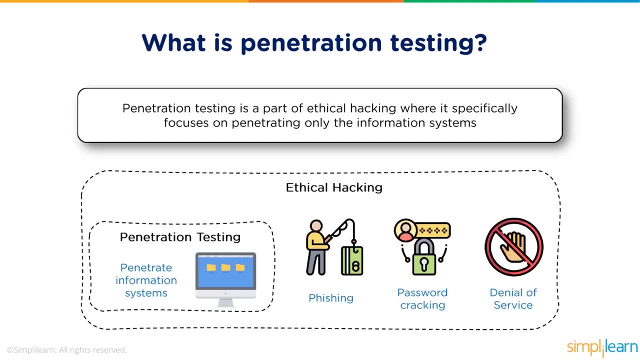 Your idea is to create those tools, create those attacks and try to penetrate into those areas where security is weak. The essence of penetration testing is to penetrate information systems using various attacks. The attacks could be anything like a phishing attack, a password cracking attack. 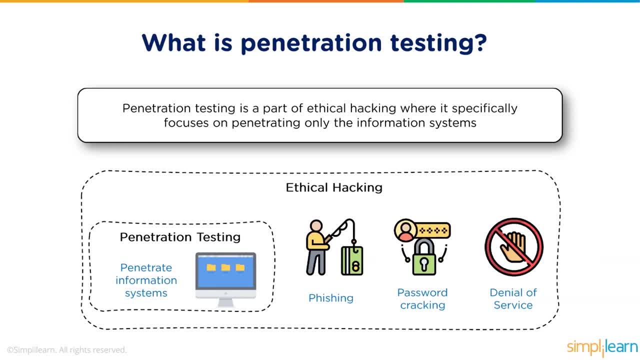 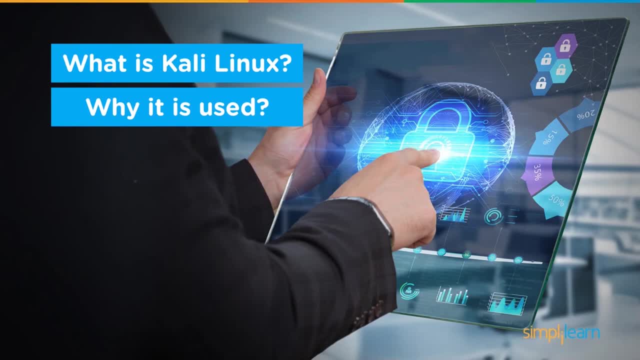 a denial of service attack or any other vulnerabilities that you have identified during the vulnerability scan. So what is Kali Linux and why is it used? Kali Linux is an operating system oftenly used by hackers and ethical hackers, both because of the tool sets. 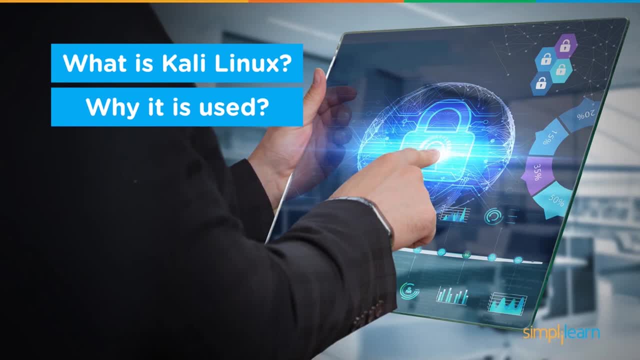 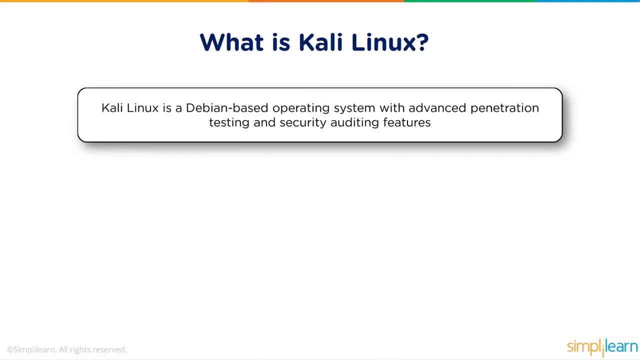 that the operating system contains. It is an operating system created by professionals with a lot of embedded tools. It is a Debian based operating system with advanced penetration testing and security auditing features. There are more than 600 plus odd tools on that operating system that can help you leverage any of the attacks: man-in-the-middle attacks, sniffing, 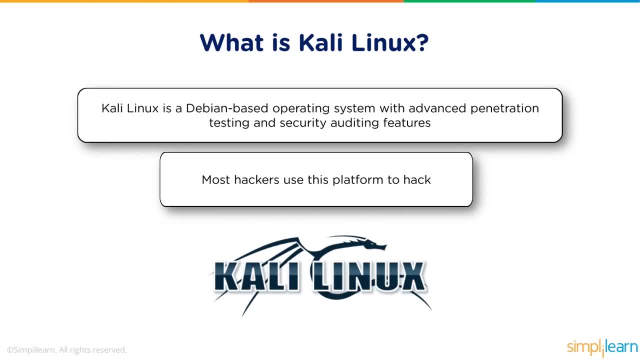 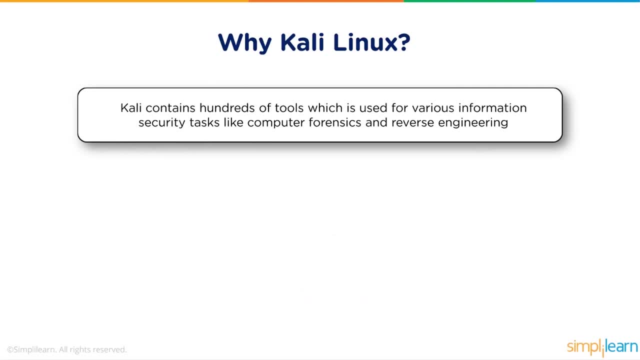 password cracking. any of these attacks It would be possible with all the tools available. You just need to know how to utilize the operating system and its tools. It contains, like I said, hundreds of tools that are used for various information security tasks, like computer forensics, reverse engineering, information finding. 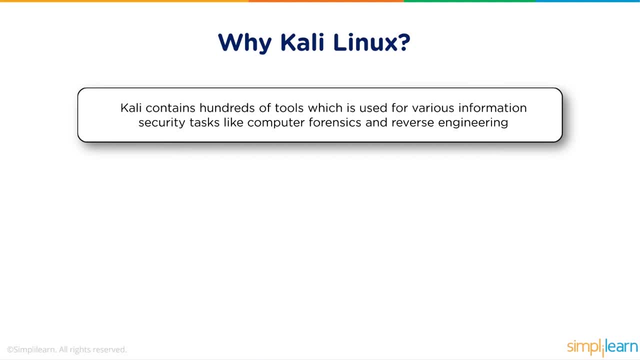 even getting access to different machines and then creating viruses, worms, trojans, anything that you will- 600 plus tools in the Kali Linux operating system. There are periodic updates that are given out to the operating system as well. It is open source. That means it is free to utilize. You can even have the source code. 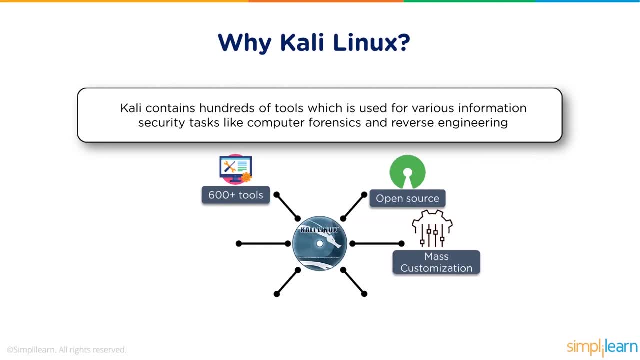 You can modify it if you want to. There's customizations available for all the tools. You can download third-party tools and install them if you want. There's a wide support for wireless network cards. Multiple languages are being supported at the same time as well. 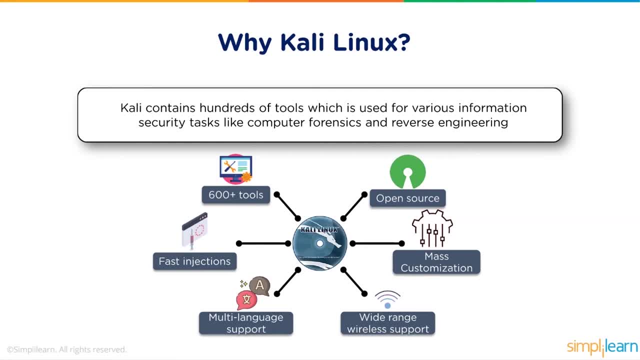 And you can create a lot of attacking scripts. You can create attacking tools and you can write your own exploits as well on Kali Linux. So this all in all helps you create a very robust system where you can create your own attacks and then launch them against unsuspecting victims. Now, that is illegal. So as far as ethical, 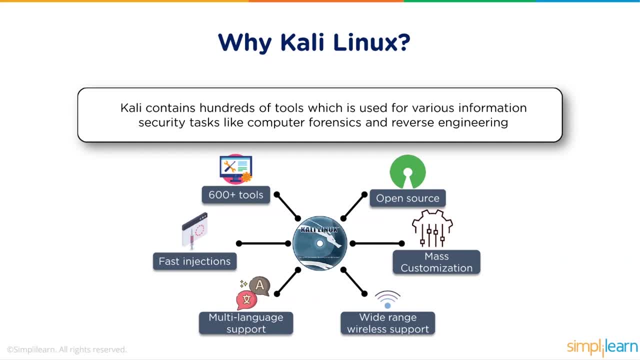 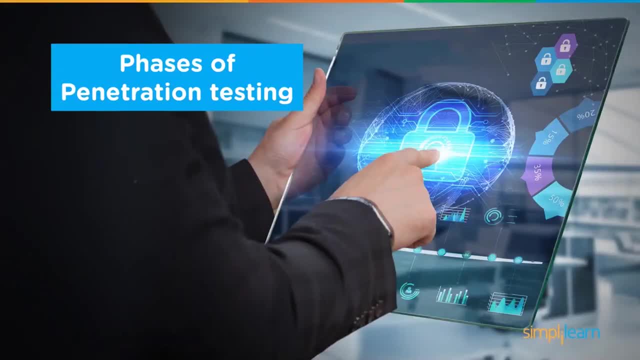 hacking is concerned. once you have authorization, you're going to identify which tools to be utilized, You're going to get the appropriate permissions and only then are you going to attempt those attacks. Let's talk about the phases of penetration testing. Now there are five. 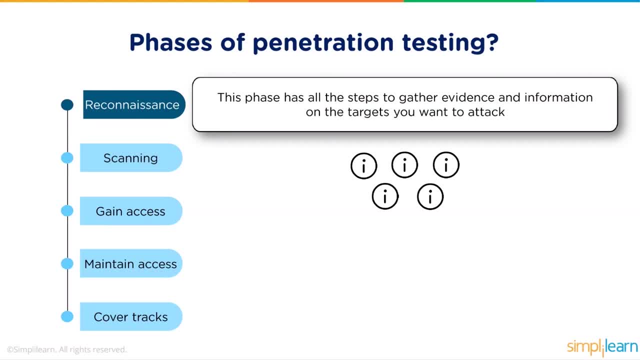 different phases. The first one is the reconnaissance phase, also known as the information gathering phase. This is the most important phase for any hacker. This is where the hacker- or the ethical hacker, if you will- will gather as much information about the target's victim or vice versa. 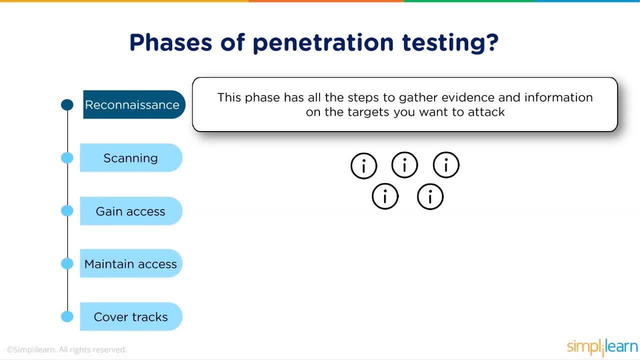 the victim. So, once you have that information, you would then be able to identify what toolsets to include and how to attack the victim. For example, you want to find out the IP addresses, the domains, subdomains, the network architecture that is being utilized. You want to identify operating systems. 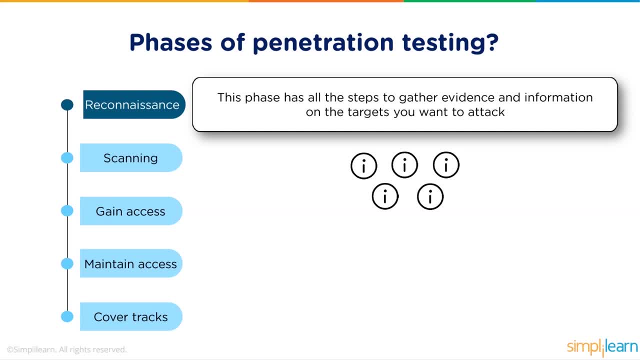 that are being utilized, the network IP ranges that are being utilized, and so on, so forth. You might want to identify employees within an organization for social engineering attacks in the future: email addresses, telephone numbers, anything and everything that will help you validate and. 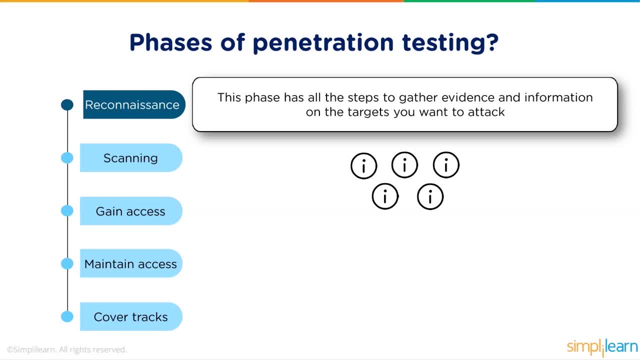 give you information about the target is something that you want to do in the reconnaissance phase. At this point in time, we are not going to question whether whatever information we are getting is useful or not. Only time will tell, depending on the various attacks that you will. 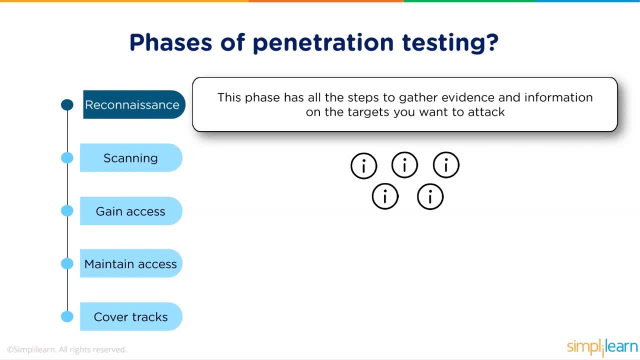 be building up later on. This becomes your baseline, this becomes your database with all the information about the victim, so that you can come back from later stages, back to the reconnaissance phase, to look at the information that you have gathered. and then you can fine-tune. 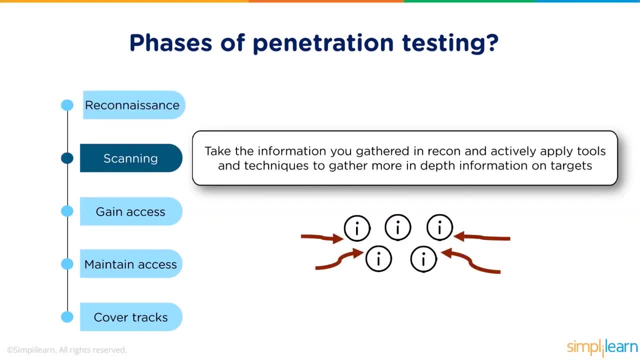 your attacks. Once you have done that, you are going to then start the scanning phase. Based on the information that you have gathered, you are going to identify live machines within the network. Once you have identified the live machines, you will scan them for open ports. 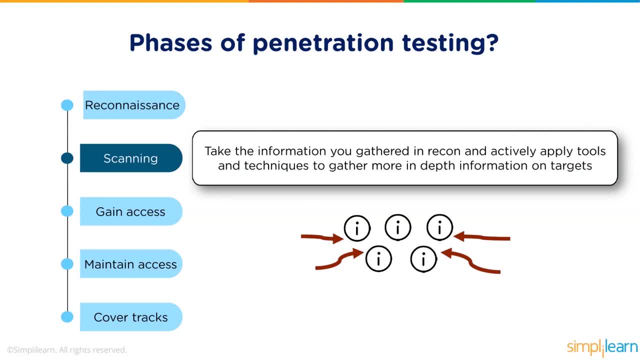 protocols and procedures, any processes that are running, and then we are going to identify vulnerabilities within these processes and within these open ports. So in the scanning phase, why do we need to find live machines? Because we want to find out the machines that have booted up, have an operating system and are running on the network. If an 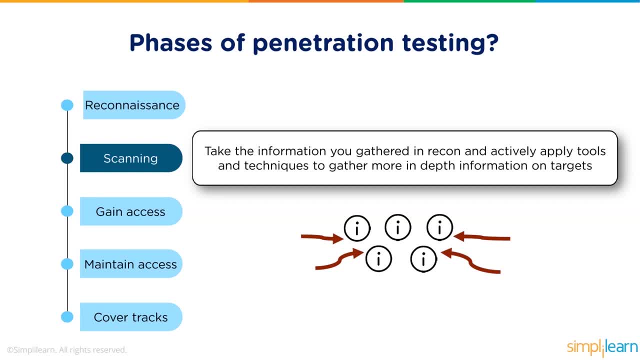 machine is not available on the network or is in a shutdown mode, that machine cannot be hacked through a technical attack, Then it would be a physical attack where you physically go to the machine and then do whatever you want to do with it. For a technical attack you will have to. 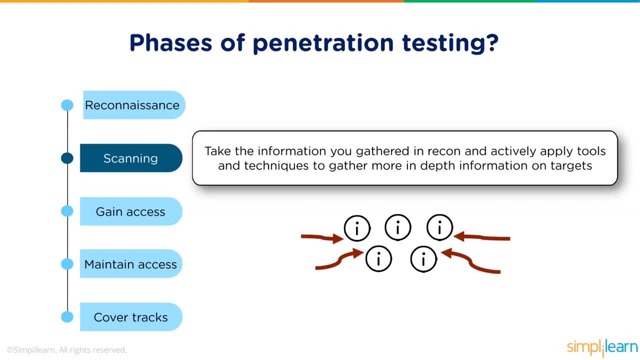 identify the machines that are running on the network and then you will have to identify the machines that have booted up. Then you are going to scan the open ports, because that's going to be our entry point And on the port would be a service that is running. So you scan the service as well. 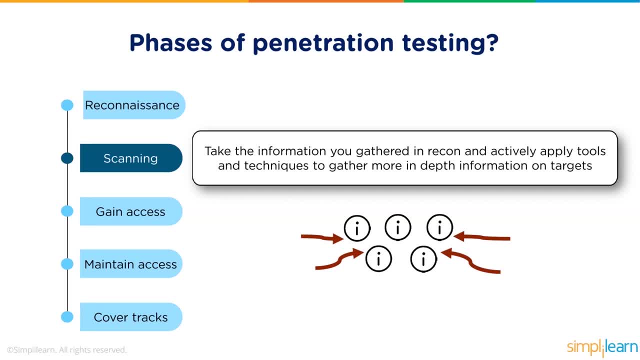 identify the version of the service and then do a vulnerability scan to identify if there are any vulnerabilities on those services that are running And then, based on all of this information, we are going to develop our attacks as we go on. So once we have this, we go on to the gaining. 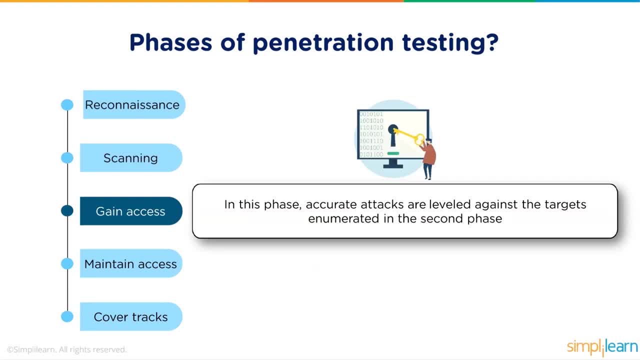 access phase, where we are going to attack and try to get access to our victims' machines, Could be a social engineering attack. based on the information gathering we have done In the technical assessment and scanning phase, if we have identified a vulnerability, you're going to. 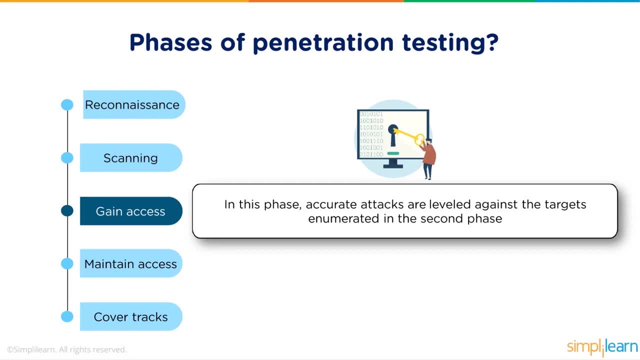 identify a relevant exploit and then use that exploit to try to gain access. Or we might just craft a Trojan and try to execute that Trojan on the victim's machine to check if we can get access through that particular manner. Once we have the access could be even a simple password cracking. 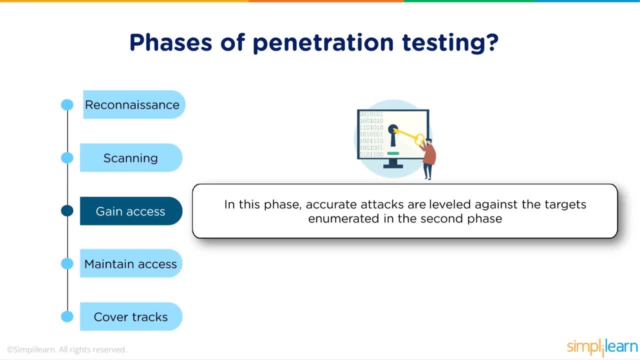 attack which we have been able to accomplish and we have cracked the password of the person and now we have gained access to that person's computer. But these attacks would be temporary. For example, we have cracked a password. Somebody changes the password every 30 days After that. 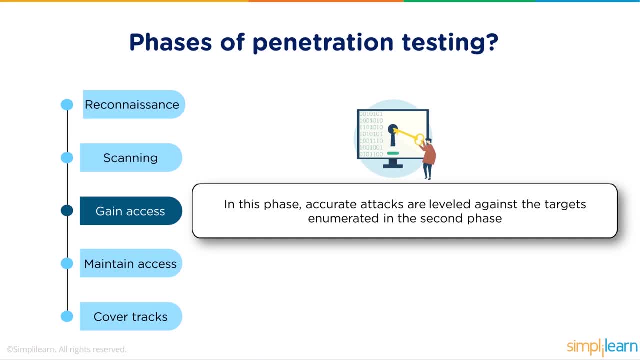 period, our attack would be useless. If a Trojan is executed, we get a connection to that machine for once, But then how do we get a repeated connection over and over again if we want to reconnect to that machine? So that's where we come into the maintaining access phase. 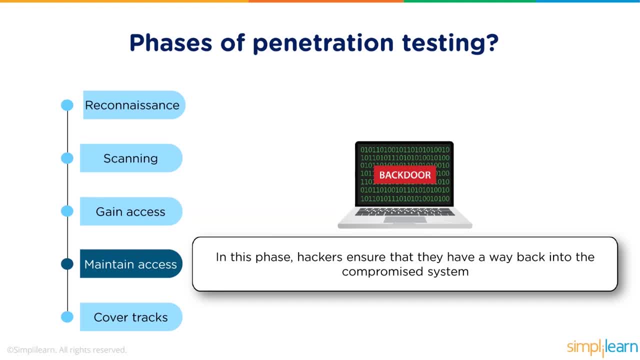 where we install rootkits, keyloggers, sniffers and things like that Where we could get a backdoor entry to the victim's machine. If we have already been successfully installed a Trojan, we would want to add the Trojan to the startup menu so that. 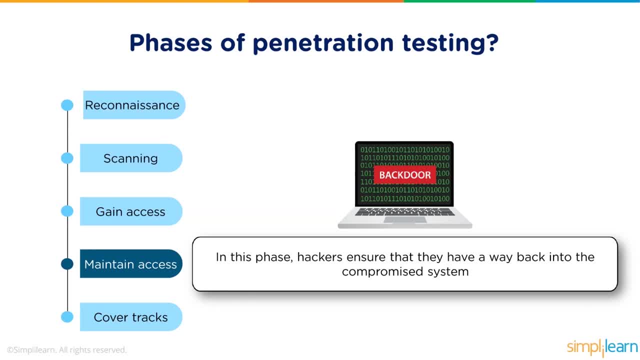 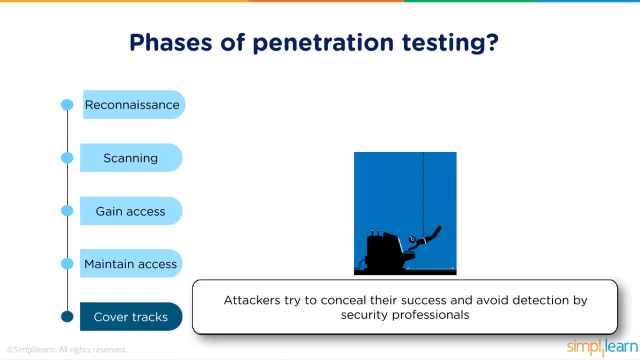 every time the operating system starts, the Trojan gets automatically executed, and thus we maintain the backdoor entry to that victim's machine. Once we have done all of this, all these activities are going to leave a trace in the victim's machine. So if we install a Trojan, a Trojan. 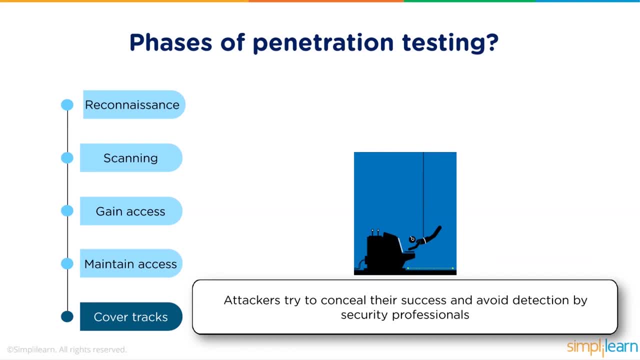 being an application, would create directories and files. A virus would be destructive in nature. If you are executing a script, it will leave some logs behind. If we even log in through the cracked password that we have, it will create a login entry for that particular timestamp, along with the IP address that we utilized In the covering. 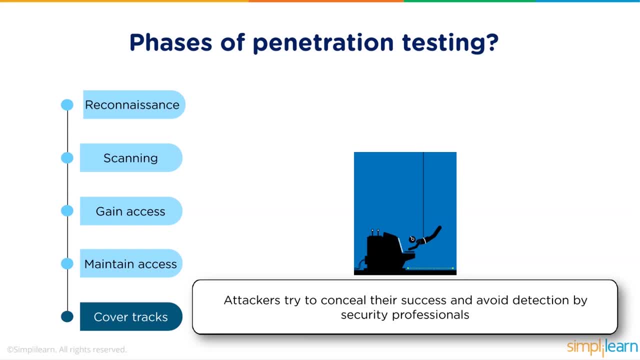 tracks. we are essentially trying to avoid detection by deleting traces of our activity. That means that we need to identify where logs have been stored, We need to address those logs and we need to delete them or modify them in such a way that our activity is not. 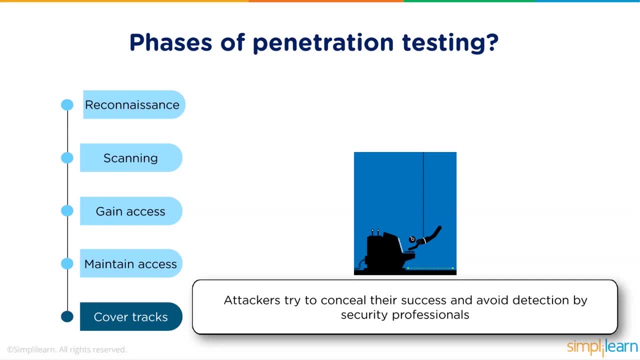 traceable. So these are the five main phases of a penetration test. Gather as much information as you can Scan for machines, ports, protocols and services running on the victim's device. Try to gain access by password cracking. Trojans. exploits for the vulnerabilities, if any. Maintain that. 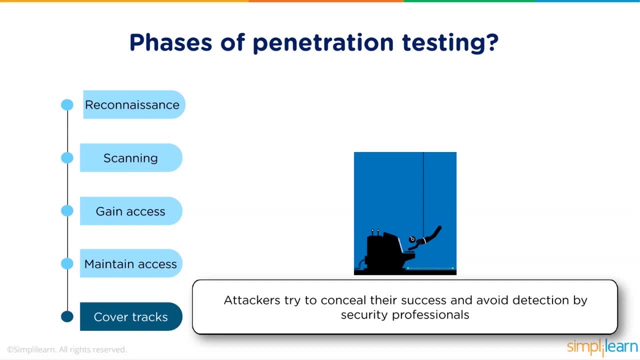 access by installing further software which will allow you to get backdoor access to that particular system and then try to cover your tracks by deleting all traces of your activity. Once successful, the victim will have no idea and you have a backdoor entry and you can. 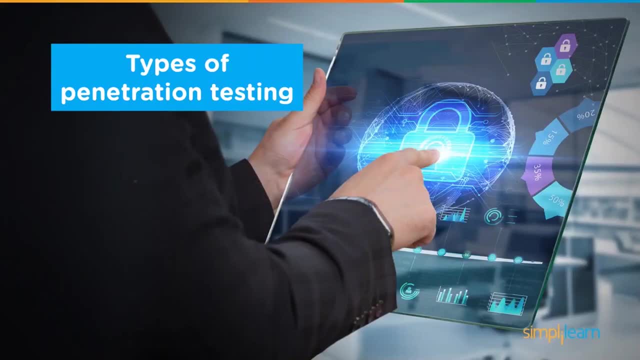 delete him to the extent that you want. Now, in an ethical hackers perspective, this penetration tests can be done in multiple aspects. So again, understand the fact that we are doing an authorized activity. We have identified the tools that we have to use, identified the attacks, We have got the appropriate. 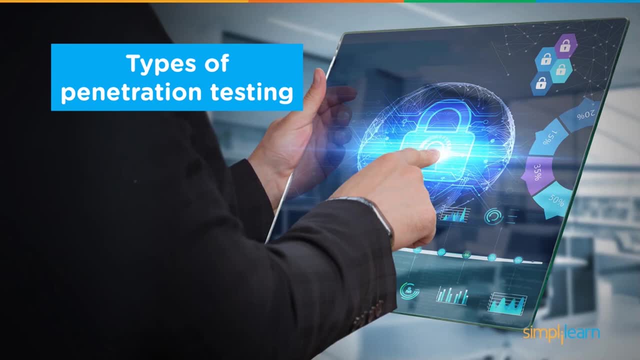 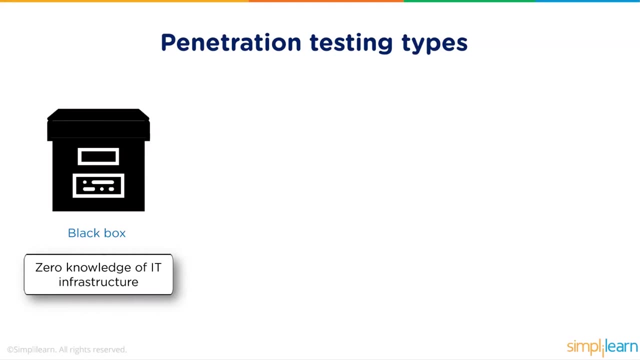 authorization and based on that authorization, we are conducting a penetration test. The penetration test may be asked to be done in one of these manners. First is the black box test. The black box test is where no information is given to the ethical hacker about the attack and the purpose of the attack and the purpose of the attack. 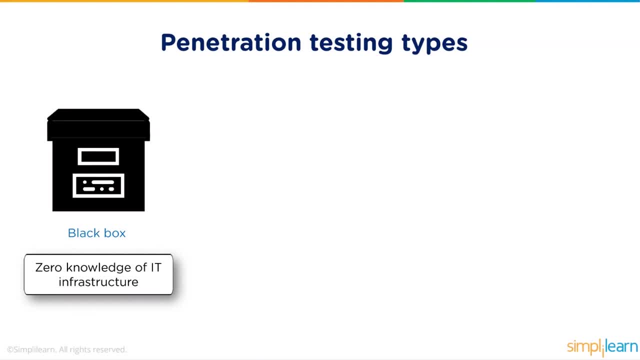 the IT infrastructure. So they have no idea what it is. they start right from the first phase of the information gathering, gather as much information as they can and based on the gathered information, they try to create and launch attacks to see if they are going to be successful. 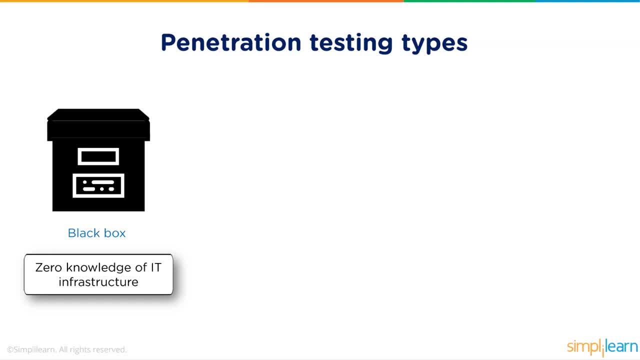 Now, not only does it test the knowledge of the penetration tester, it would also test the security implementations that the organization has done to see whether they can identify the attack and prevent it in the first place. So this is a simulation of a malicious hacker scenario. 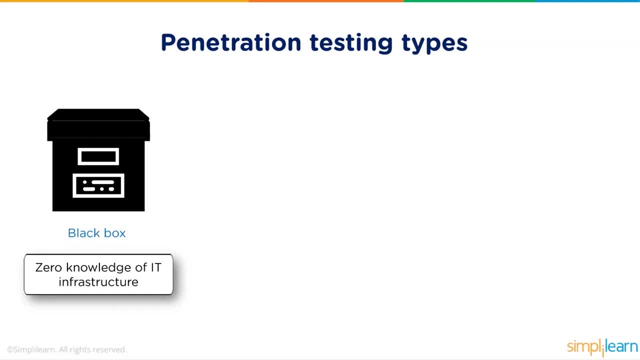 where a malicious hacker, having no idea about the organization, first tries to gather information and then tries to attack that organization. So no source code knowledge, no technological knowledge, nothing. They're just going to try to gather information, scan those devices and then try to gain access. The second test is a gray box test, where some information is given or some. 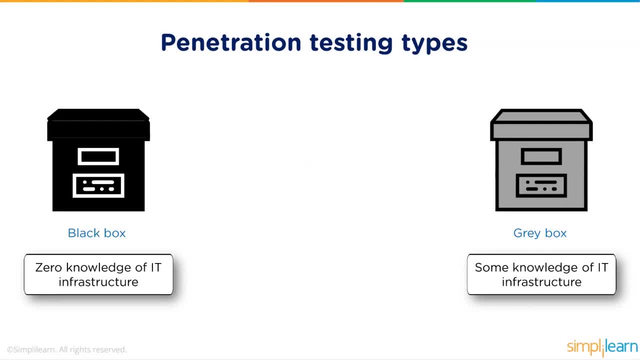 knowledge of the IT infrastructure is given. Think of it from a employee's perspective. A regular employee in an organization who doesn't have extra privileges like an administrator, but it's just a regular employee, does that means that they were limited access within the organization, based on which they get some knowledge of the IT infrastructure? So this is an attempt of 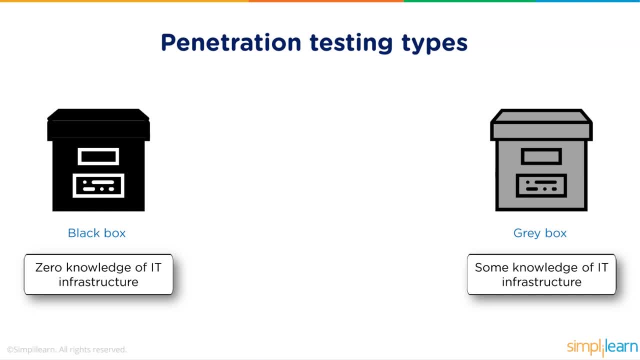 an insider simulation attack, where a regular user may want to try to misuse the access that they've been given and then try to gather information or try to gain access to other devices which they are not authorized to. The third test is white box, where there's full knowledge of the IT. 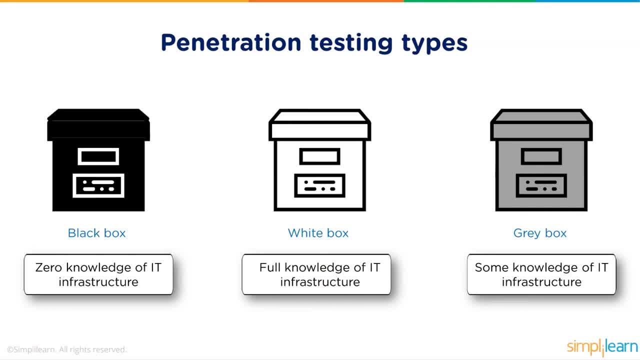 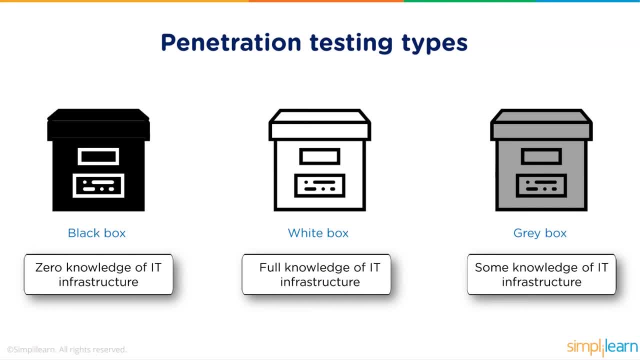 attack a malicious insider, if you will, but at this point in time the person has complete knowledge of the infrastructure, could be in an administrative position, and then they are trying to leverage their access to see if they can get information or they can compromise any of the data. 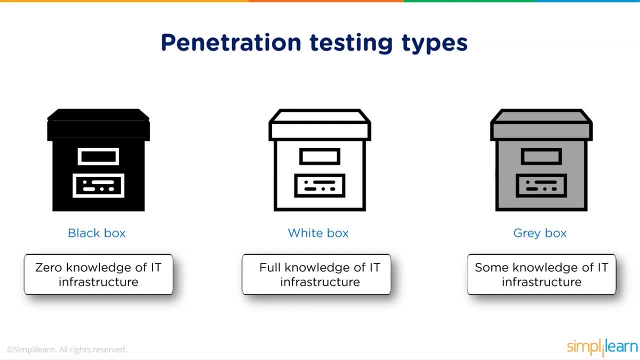 So the three attacks would be: the first one, black box, where we are simulating an external threat, a hacker sitting outside the organization trying to gain access. The gray box is an insider threat, where there is a regular employee who is trying to get access to infrastructure. 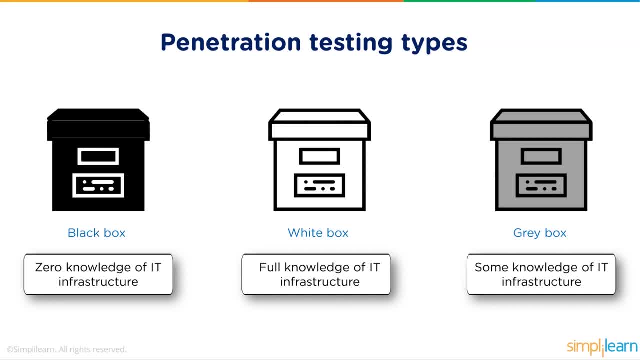 that they are not authorized for. and then the third audit is a white box audit, where there's an administrator who has all the leverage, all the access and the visibility within the infrastructure and then they are trying to misuse their access to see what else they can get from. 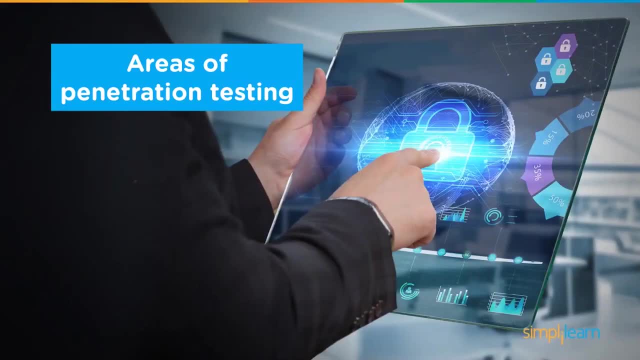 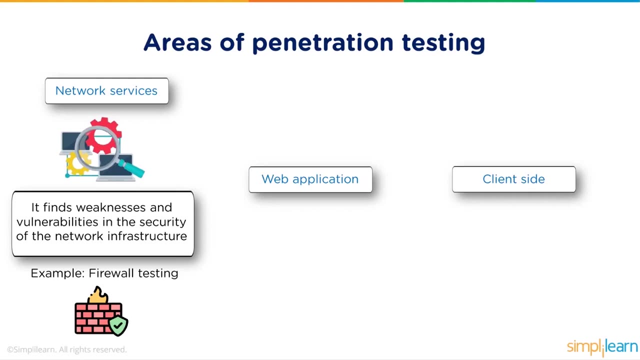 whatever access has been authorized to them. Now let's look at the areas of penetration testing. where all could we do a penetration test, thus compromising the security of the application or of the server or of the user? So, first and foremost, network services, it finds. 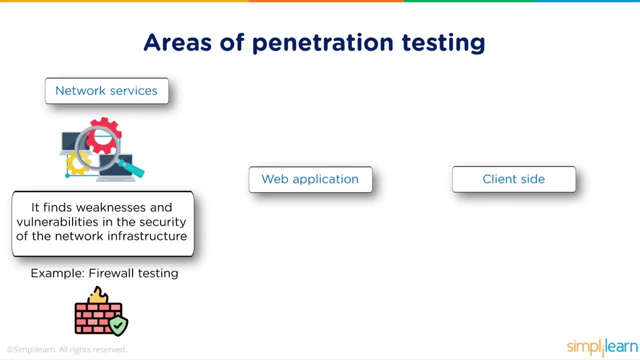 vulnerabilities and weaknesses in the security of the network infrastructure. So, for example, we have switches, routers, firewalls in the network. All of these are devices that need a configuration If they have been not correctly configured or if they have not been correctly. 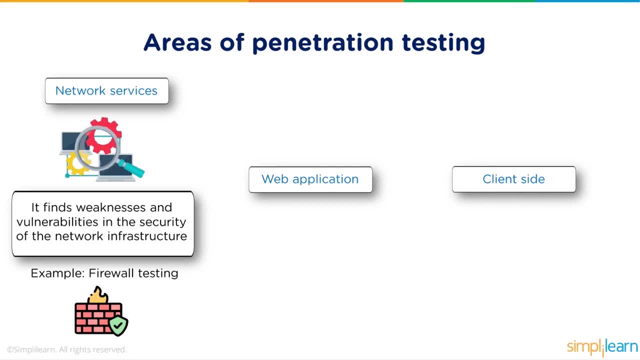 secured, they would leave some vulnerabilities behind. If we, as ethical hackers, are able to identify these flaws, these misconfigurations, these vulnerabilities, we could then try to exploit them and try to gain access to the network and devices within that network By getting access to the network in the first place. Then we have the web applications. 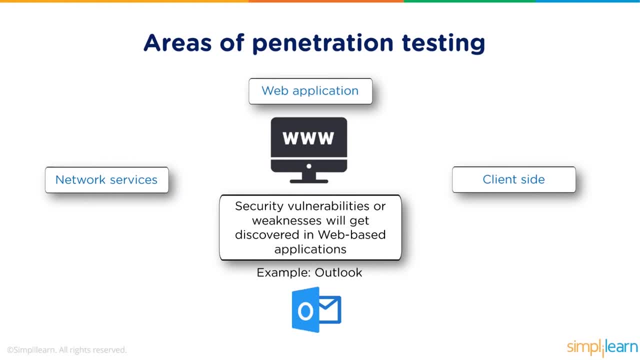 Web applications are nothing but softwares that are developed over or deployed over a web server and are made available over the intranet or the internet, For example, websites that we visit or web applications like Facebook, if you will right. So if these applications have vulnerabilities, 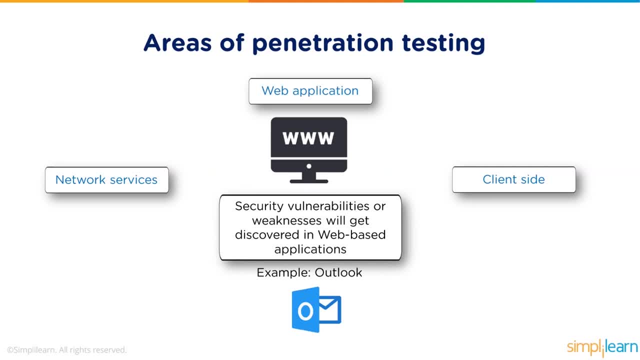 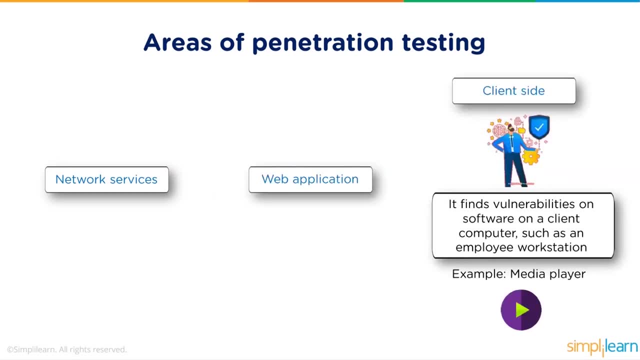 within them. we then try to attack the web-based applications and thus try to bypass authentication or get access to database or try to leak information through those applications. If not, then we try to attack the client side. Now web application is at the server level and 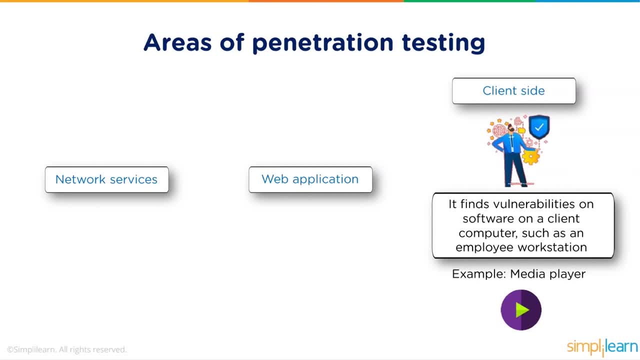 is hosted by the deployer, So that's at the server side. The client side is where we, as users, are using a computer with a browser and trying to interact with the web application. Now, the browser and the operating system that we are utilizing would have its own vulnerabilities. Thus, 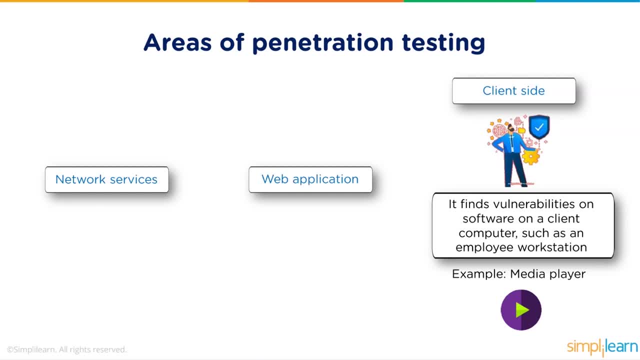 identifying a client side vulnerability and then exploiting it to either either hack the client or then piggyback on the client's connection and try to get access to the server. So either you could attack the network, the web application or the client side itself, Or you could attack wireless. 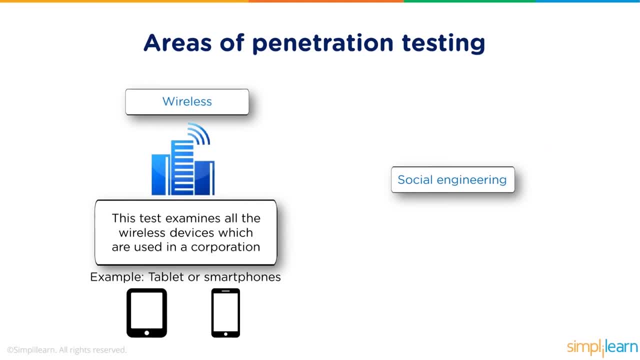 networks. This test would examine all the wireless devices which are used in a corporation. Most of the wireless would have laptops, smartphones, tablets, phablets- all of those connected to them. If you are able to access any of these devices through the wireless, it would help you. 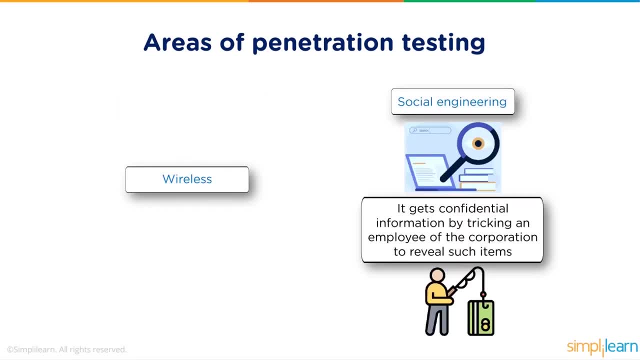 gain access to other devices on the wireless as well. And then social engineering. So this is where you are trying to attack humans. You are tracking an employee of a corporate corporation to reveal some confidential information, knowingly or unknowingly, by tricking them with fake mails or fake websites or malicious emails that you have sent to them. 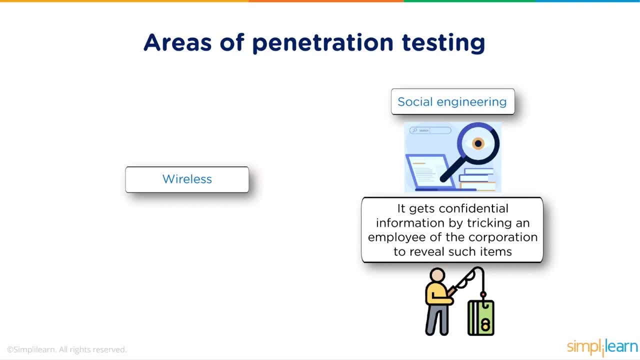 which they have failed to recognize as malicious and they click on it, thus getting victimized. Social engineering attacks are always successful because of the gullibility of humans: Empathy, sympathy. Humans basically have emotions. Emotions can be toyed with and then taken advantage of if 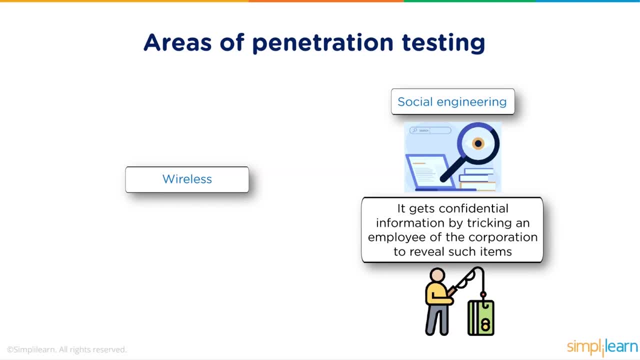 the person is not careful. Now, for example, the most common social engineering attack that we see is the Nigerian fraud, where we receive an email that someone somewhere has died and has left a huge estate behind a few hundred million dollars, and we have been identified as the person through whom they want to. 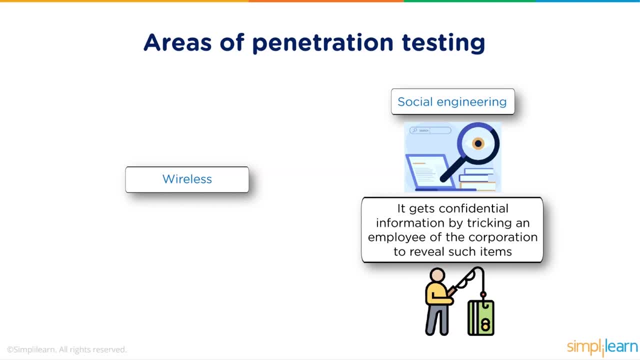 transfer the money to a foreign land to save on taxes. What are the chances of that happening on a daily basis, Right? How many princes are there? So that's something that we do not verify. It's just the- I guess the greed, if you will, of striking it rich quickly. 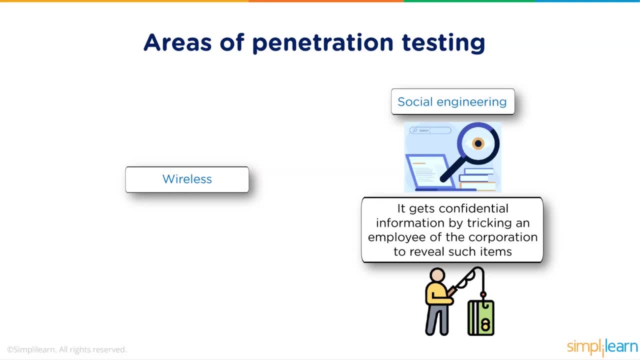 that makes us believe these kinds of emails. We have also received emails of lottery tickets that we have won over a period of time without even having bought a lottery ticket. So if you haven't bought one, what did you win? But we don't ask these questions. We just get excited about the 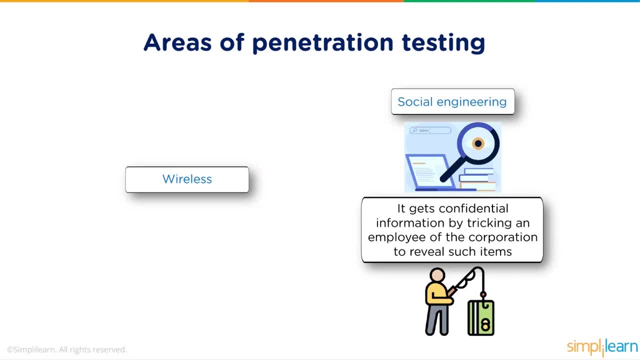 amount of money that we have won, and then we try to bet on our luck and try to see if that email is going to fructify. or is it just another scam? So social engineering attacks are dime a dozen these days and we need to be very careful on what we trust on the internet. Let's look at the penetration. 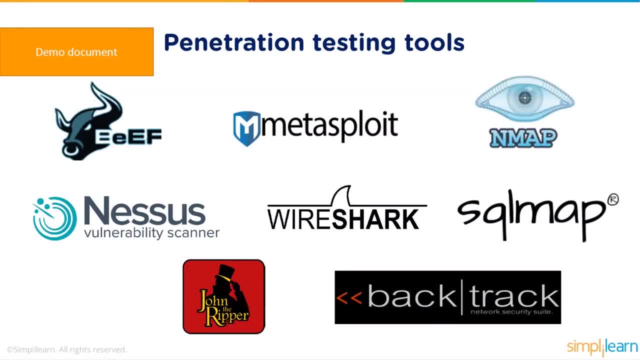 testing too. Let's look at the penetration testing too. Let's look at the penetration testing too. There are hundreds and thousands of tools out there. Most of these have been concise and collected together and hosted on a operating system known as Kali Linux. that we 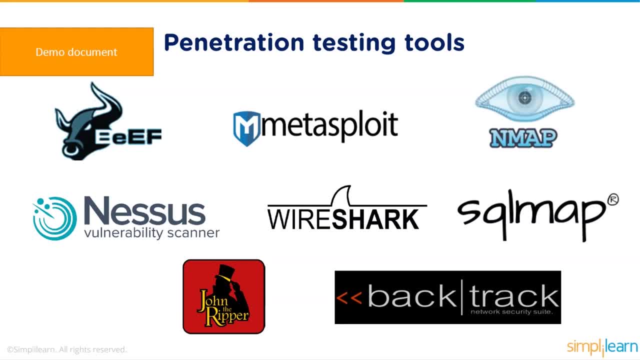 have talked about earlier. Now, the predecessor to Kali Linux was Backtrack. Backtrack is no longer continued. It has been discontinued, and Kali Linux has taken the place of Backtrack, within which are all the tools that you see on your screen. Metasploit is one of the most favorite. 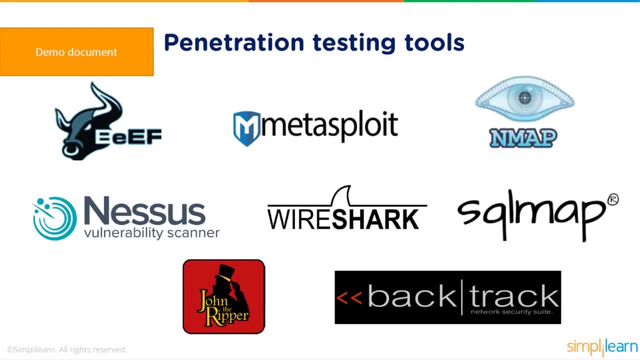 penetration testing tools of hackers and ethical hackers. There are a lot of inbuilt exploits over there and we'll be doing a demo at the end of the session on this. Nmap is the information gathering tool which will scan for live devices, scan for open ports, protocols and 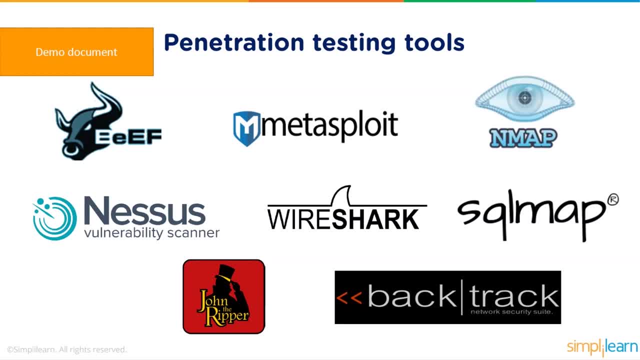 services. Beef would be an application testing tool that would help us find exploits within applications. Nessus Vulnerability Scanner is a network and host-based scanner that would help you identify vulnerabilities within such hosts. Wireshark is a network sniffer, which allows you to capture. 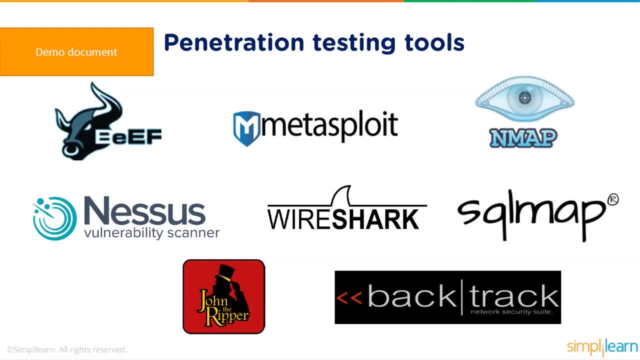 network packets and and analyze them to see if there are there is any information worth capturing within those packets. sql map is a automated tool used for sql injection attacks. so you don't even have to craft your queries for sql injection, it will be done by the sql map tool. you just need to identify whatever. 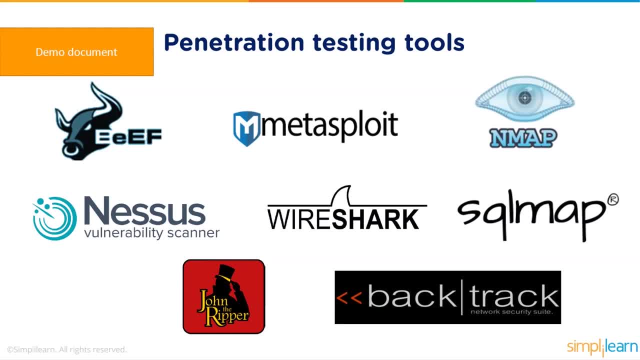 is possible through the queries that the sql is going to create. and then, based on the activity that you've identified, you just need to redefine your search parameters to get access to the sql map, or sql map as well. and then there is john the ripper. john the ripper is a tool that 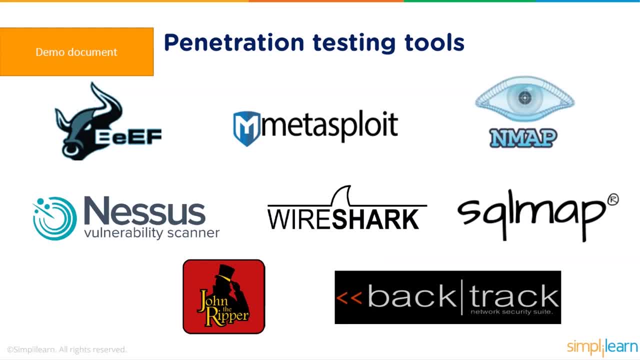 is used for password cracking. so dictionary attacks, brute force attacks, are done using john the ripper. what is a dictionary attack? a dictionary attack is an attack where we create list of all probable passwords, store them in a txt file and run that list against the password tool to see if any of those passwords are going to match. a brute force attack is trying the same. 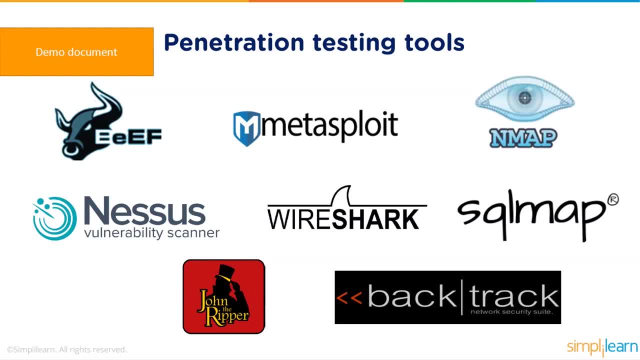 attack, but with every permutation and combination of the alphabet that we have, and we're going to try to figure out if we are able to crack the password at all. so these are just some of the tools. for every tool there are another supporting 100 tools or more than that. 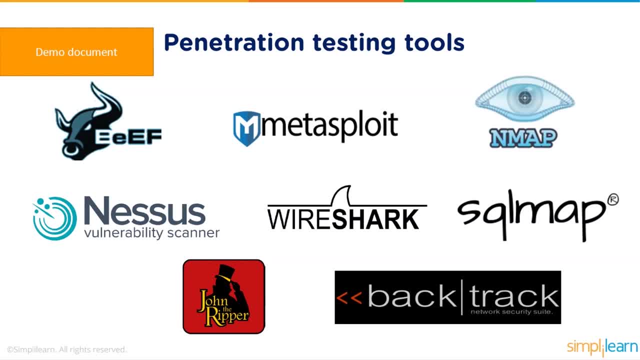 like for ness's vulnerability scanner, you'll have call this vulnerability scanner. you have gfi lan card and there are other, lots of other softwares out there, but these are some of the most commonly utilized tools. let's look at the metasploit attack. metasploit is a framework of 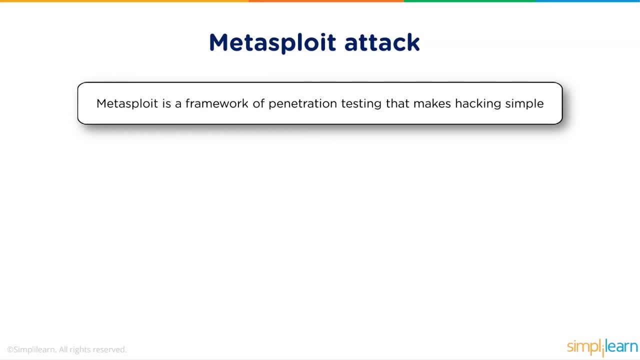 penetration testing. that makes hacking very simple. you just need to know how to utilize the tool. you can use the vulnerability associated with a particular exploit and then run the exploit on metasploit. we'll be demoing this during the practical. so there are active exploits and passive. 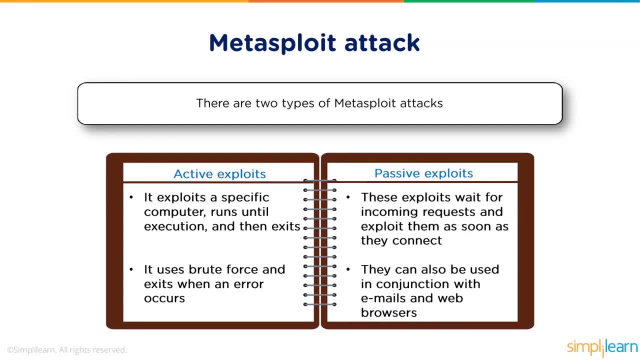 exploits. inactive exploits exploits a specific computer runs until execution and then exits, uses brute force and exits when an error occurs. in a passive exploit, these exploits wait for incoming requests and exploit them as soon as they connect. they can also be used in conjunction with emails and web browsers. so in passive exploits we create a payload. we 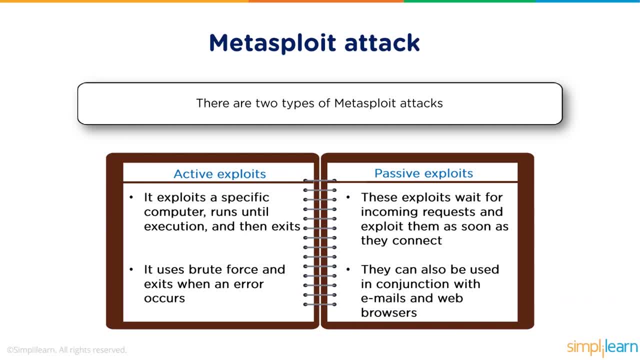 like a reverse connection payload. we send it to the victim. once the victim installs that software, the machine will then initiate a connection to us. our machine will be in a listen mode and then we will. once the software is executed at their end. we would then try to 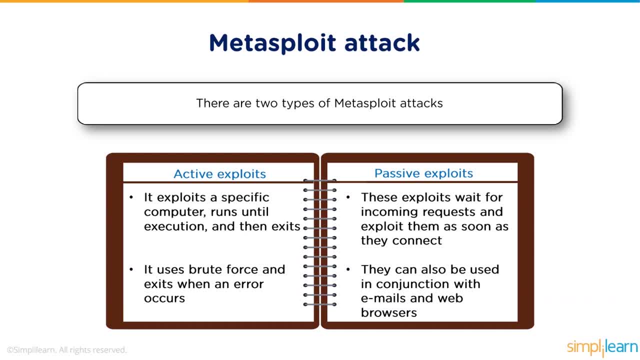 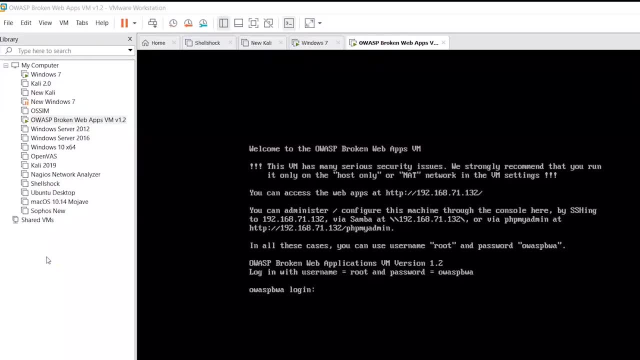 connect and exploit that particular vulnerability. this is the practical that we'll be doing on metasploit, so let's move on with the demos, and then we'll see what we can discuss amongst them. all right, let's have a look at some of the demos that we had talked about in the ethical hacking. 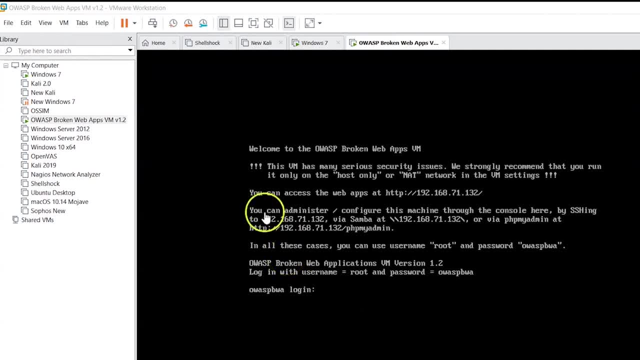 testing module. we are going to look at three different demos. the first one is going to be a sql injection attack that we are going to perform on this tool that we have. the second one is a password cracking attack on windows 7. and a third one is a meter breeder based or a metasploit based. 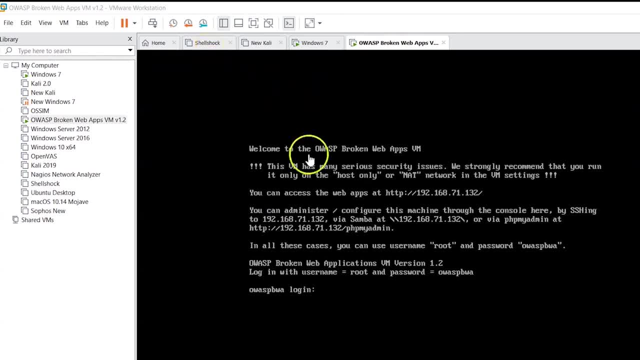 shell shock attack on a linux based web server, so let's get cracking. i've powered on this virtual machine, uh, which is the ovass broken web application. it is a tool that is provided for people who want to enhance their skills, and they can practice, uh, how to do the 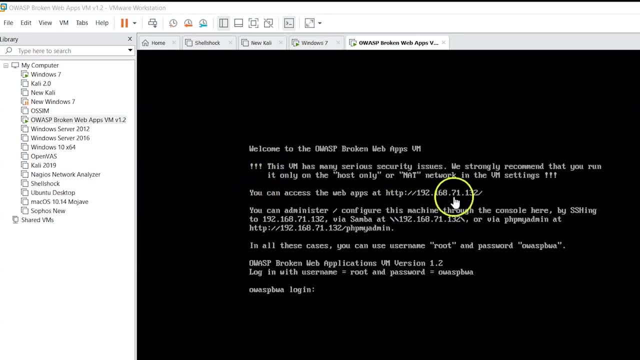 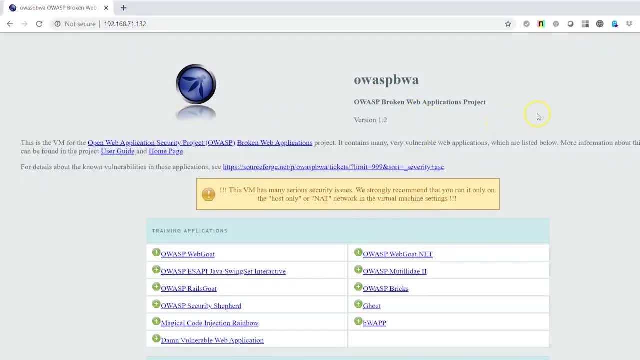 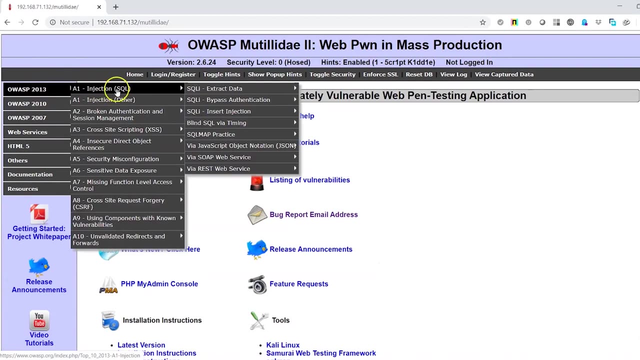 attacks in a legal manner. so we are going to go to this site. i'm just going to open up my browser. the ip address is 71.132 and that's the ovass broken web application that we want to utilize. we are going to head off to mutility day 2 and we are going to look at a sql injection attack. 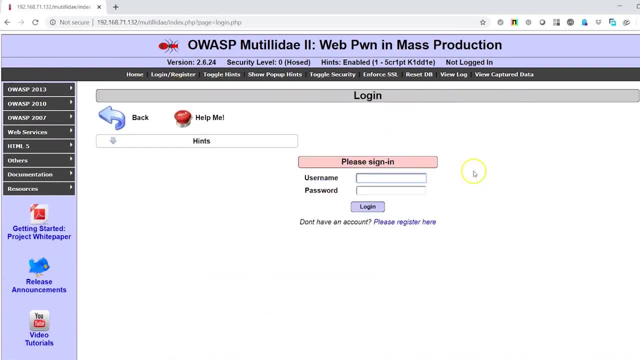 where we want to bypass authentication. now this takes us to the login screen, so we can just try our luck here and see that the authentication mechanism works. the account does not exist, so password that we have supplied is not the correct one, so we want to ensure that there's a sql. 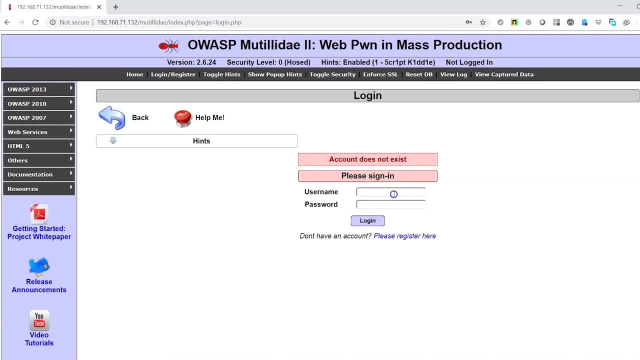 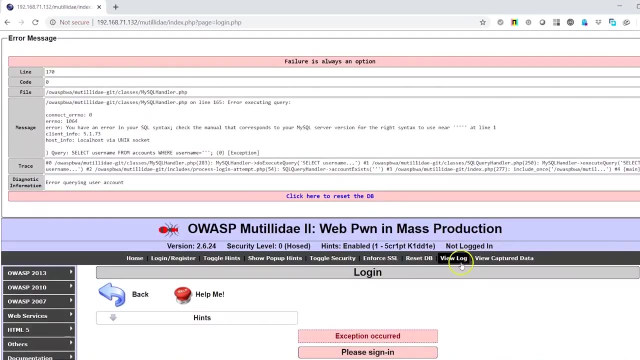 database and we can try to attack it and see if we can bypass the authentication. now what we want to do is we want to create a sql based malform query that can give us a different output. so i'm just going to type in a single quote over here and type login, and you can see that this is now suddenly. 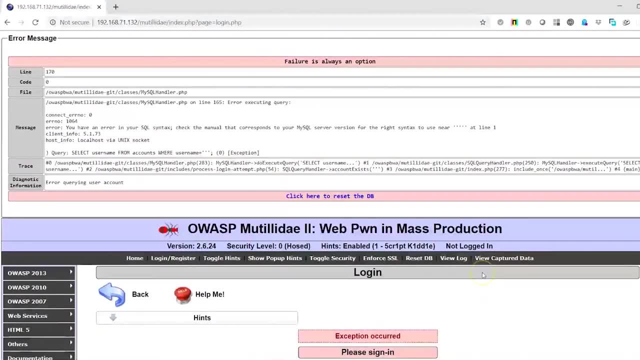 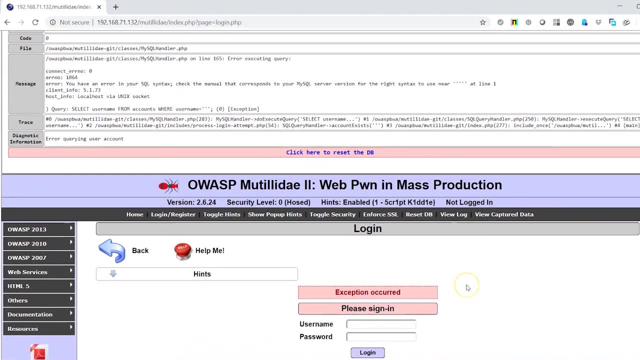 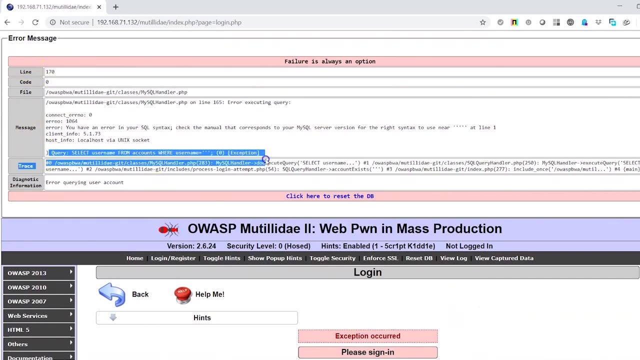 recognized as a operator and there's an error that is given out. compared to the login that we tried earlier, when we used a proper text-based login mechanism, it gave us the account does not exist, but here the single quote gave us a error and it shows us how sql works. this is the query. 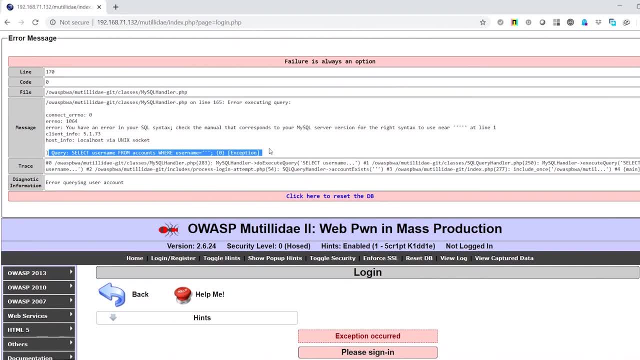 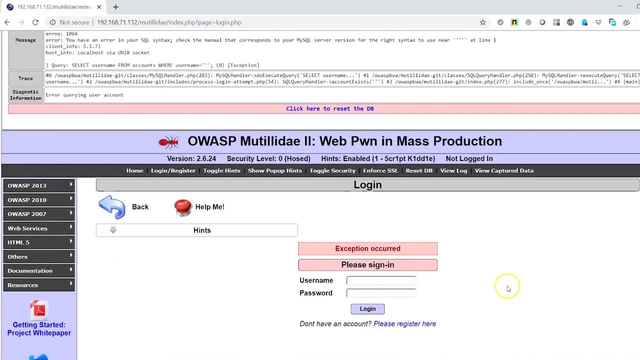 that we had created. now, in the trainings that you have for ethical hacking, there would be explanations of what these queries are all about, how this syntax works. here we're just going to see if we can create a malform query to log in as a user in this case. so what i'm going to do is create the 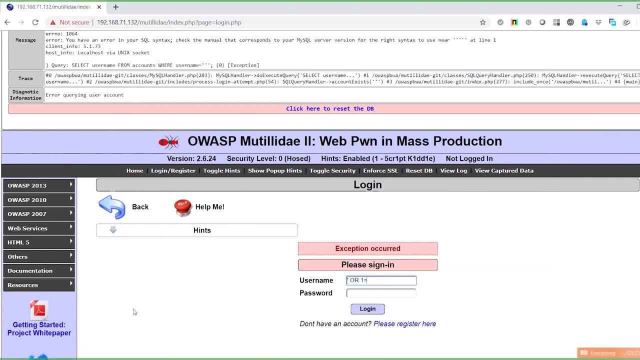 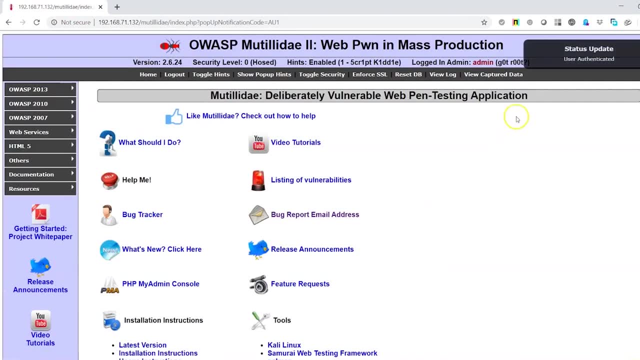 sql query and we're going to give it a comparison. so we're going to give it a or one equals one space, hyphen, hyphen, space, and if you now click login, you should be able to bypass authentication and you can see user has been authenticated and we now have admin access to this application. now, 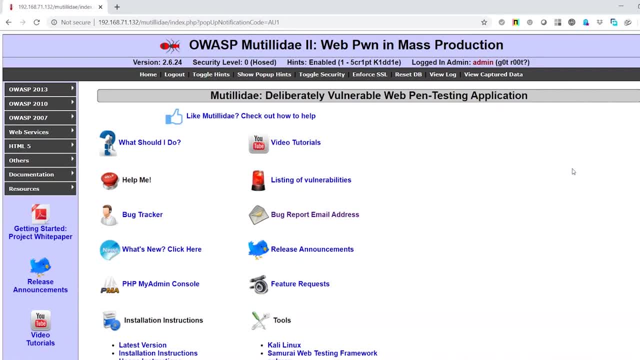 here. the sql queries need to be crafted in such a perspective that they're going to work. so there would be a lot of exercise in identifying what the database is. there's a microsoft database and oracle database and so on, so forth, and then you have to choose those proper commands. 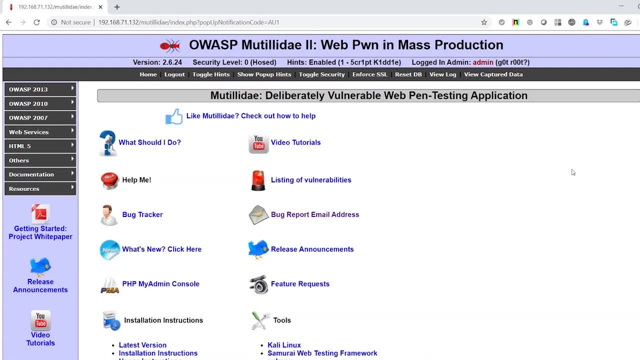 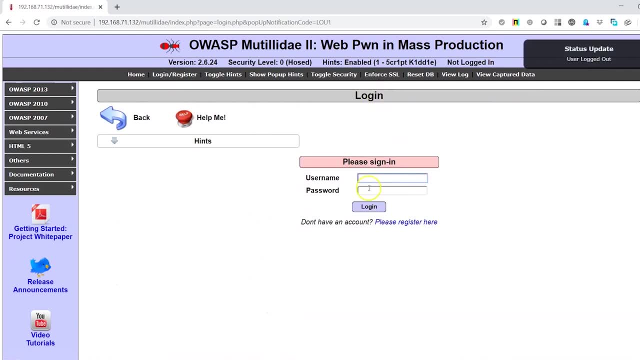 but identifying. that would come in the training. right now we're just looking at them at a demo. this is how a sql injection attack works. now let me log out here. similarly, now we are in a login page. the same query work wonders where it allowed us to bypass authentication. so it also depends. 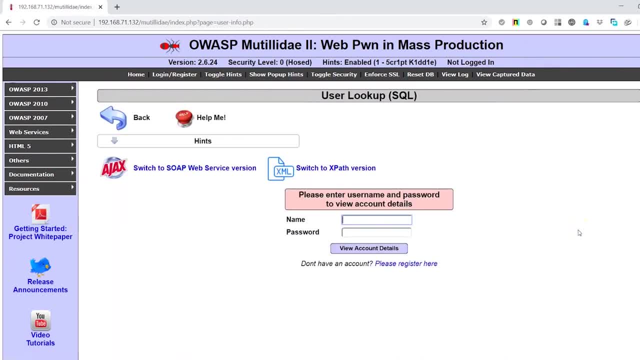 on what kind of a page i am and what query would be accepted at this point in time. so here application understanding would also come into the picture where which function we are calling upon when we are connected to a particular page. now this is a user lookup function. 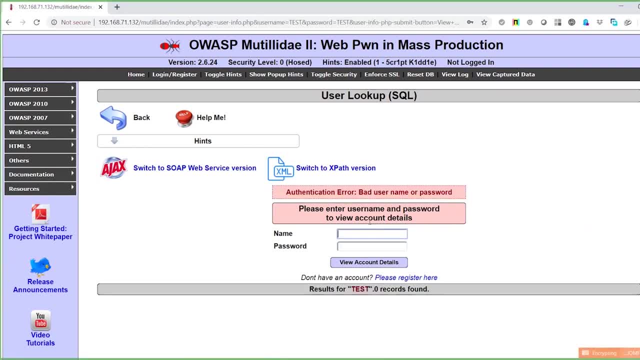 so again here we try the same method, test, test. that's not going to work. authentication error, bad user on password. and if we type in the same query over here, single quote, or, and give it a condition: single quote or one equals one space, hyphen, hyphen, space. now, here it is not going to. 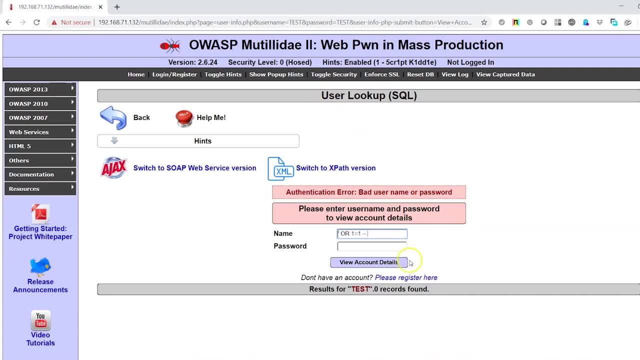 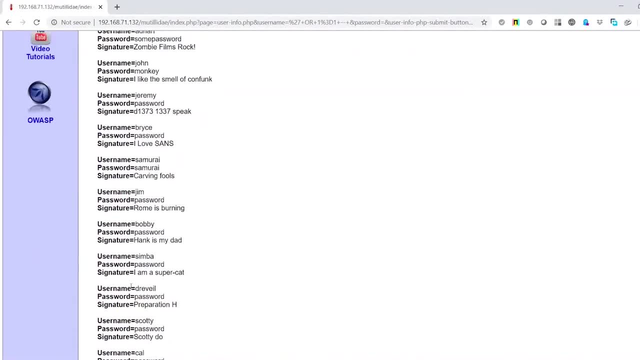 log us in, because this is not a login page. this is a user lookup form. so here it will instead give us a dump of all the databases that it has, so you can see all the user names and passwords coming in that are stored in the user lookup field. 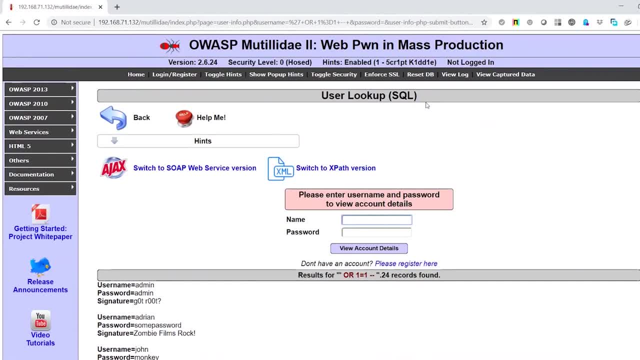 so this is where the understanding comes in of which query to create, at what page we are depending upon the function that has been called right? so that's the sql injection attack that we wanted to look at. let's move on to password cracking now. this is a windows 7 machine that we have. 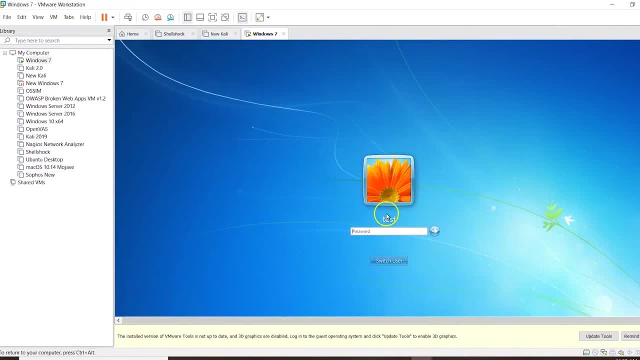 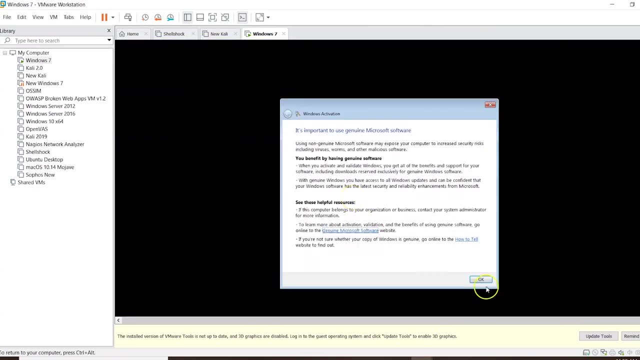 i'm just going to do a very basic password tracking example. we're just going to log in now. here, the assumption is that we are able to log in. we have access to a computer and we want to check out other users who are using this computer and see if we can find out their. 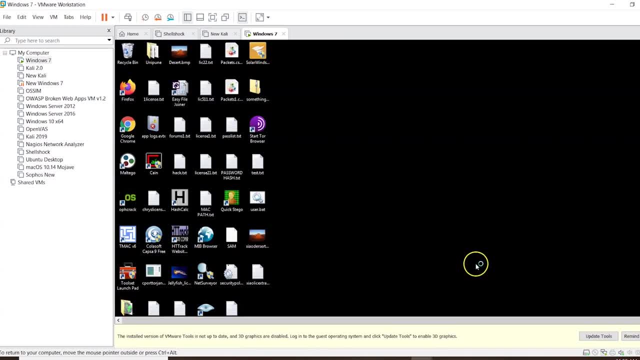 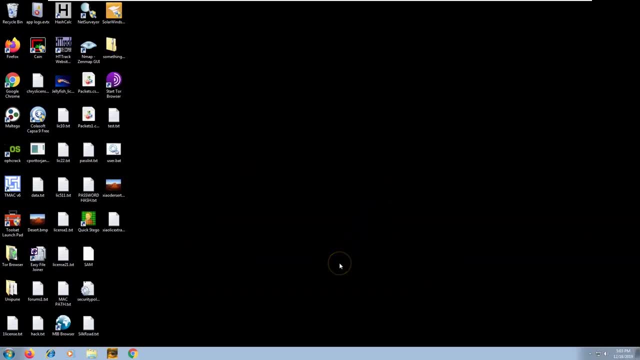 so that we can log in as a different user, steal data if required, and we wouldn't be to blame if there are any logs that are created. so here we've got a tool called kane enable that is installed right here now. i'm already an administrator on this machine and checking out other administrators. 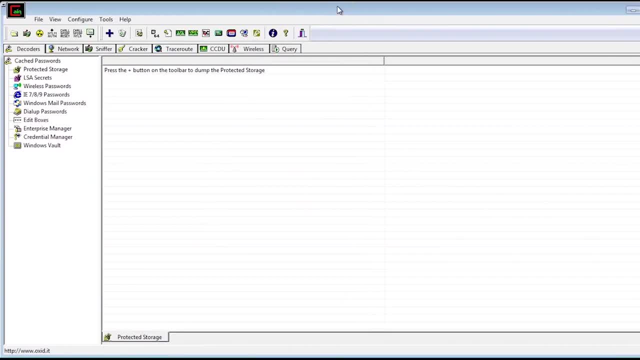 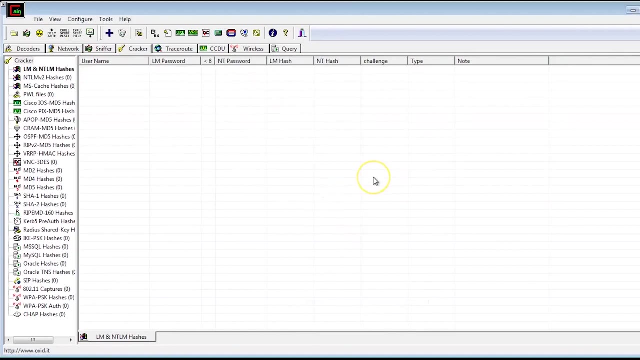 who share the same privileges, or any other user who may be on this system whose password i can crack, and thus i would be able to get access through their account and then do any malicious attacks and so on. so i'm going to click on this tool and i'm going to go into a cracker tool. 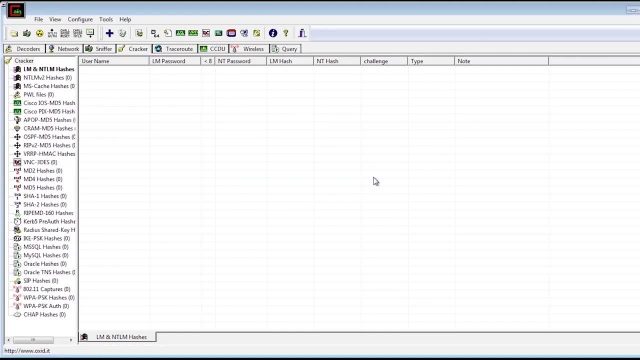 and it allows me to enumerate this machine and identify all the users and passwords that are there in this particular machine. right, so i'm just going to click on the plus sign and i'm going to import hashes from a local system. so where are these files stored? where does windows store its? 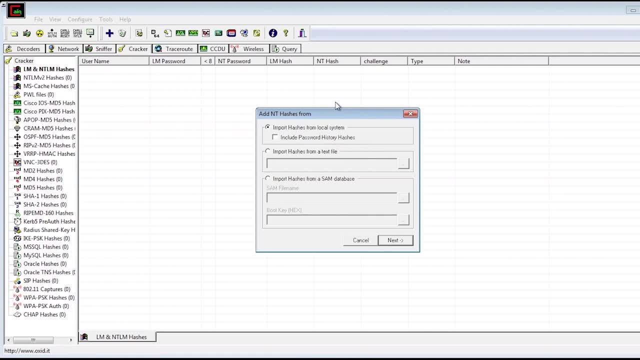 passwords, in what format are they stored and what this tool does to retrieve those. that's something that we all need to know as an ethical hacker, right so on. next, it's going to enumerate that file and it is going to give you a list of all the users that 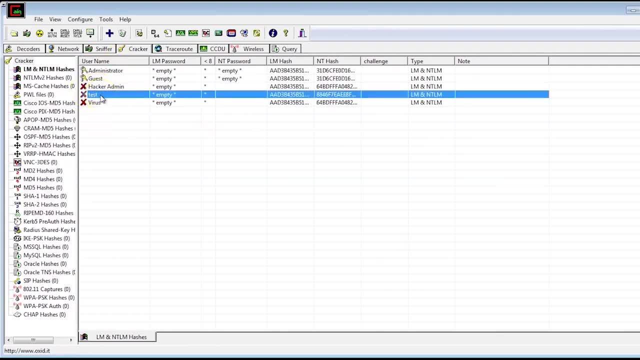 are there so you can see the users are hacker. admin test the one that we are logged in as, and then the user called virus as well, and you can see that this is the hash value of the password that is being utilized. now there's a particular format for the hash value for windows and how it stores. 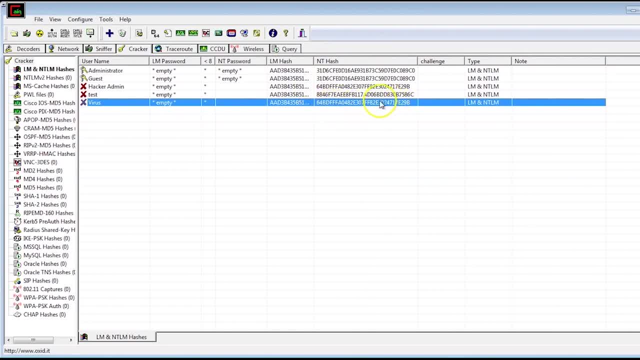 but once we have these hash values, let's say, if i want to crack this password, there are various attacks that we can do, for example, a dictionary based attack or a brute force attack. let's try a brute force attack right. ntlm is the hashing mechanism that is used by windows, so we 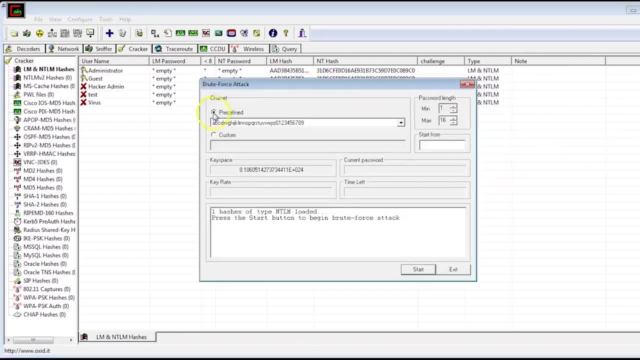 are going to try to create an ntlm hash attack, and here we are going to use a predetermined rule set, for example. we are not sure what characters are being utilized over here, so we just create an attack like this, using all characters and uh, lowercase a through z, uppercase a through z. 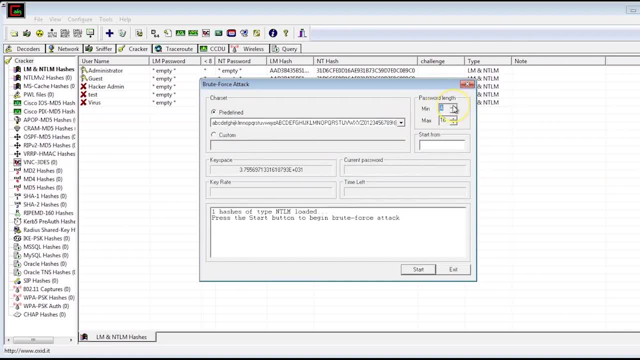 numeric 0 through 9 and all the special characters. let's say, the password is between 16 characters and this is the character set that we want to try. the brute force attack on what is a brute force attack? it is an attack where the computer is going to try each and every. 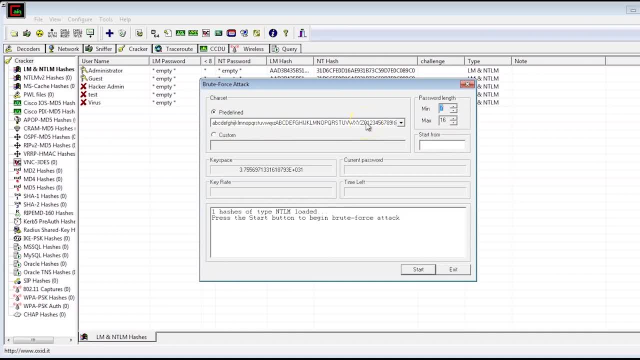 permutation and combination out of this character set and try to figure out if the password is going to be correct. so if we click start, it's going to start with a particular characters and then it is going to identify if that ntlm hash is going to work against this character and you can see the 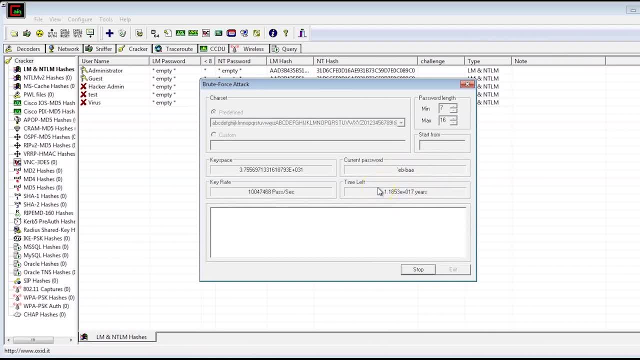 time is going to be phenomenal over here, so it's not necessary that this attack would be viable. it will be 100 successful, given the time frame. however, the time frame is huge enough for this attack to become a little bit redundant. there are other attacks that we can do, which can easily. 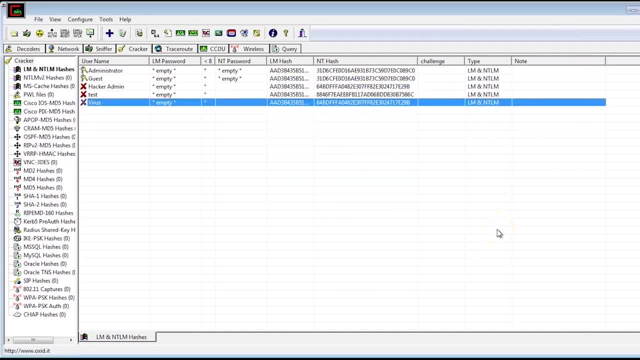 identify this data for us as well, but that is something that we will look on in future videos. so that's how we can get access to users and passwords. uh, there are different mechanisms where, let's say, we don't have login access. then what are we going to do? how we can create a fake? 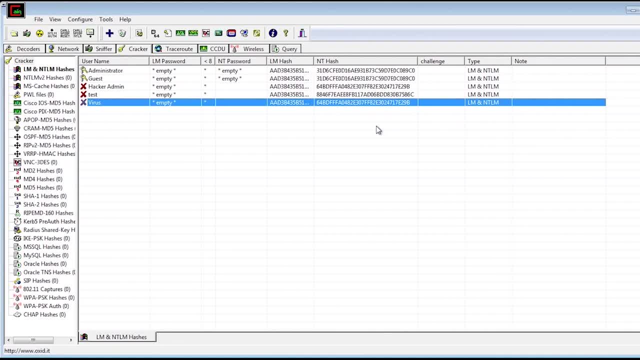 user login, or how we can remotely access a machine and then try to get the same access, and that is what we are going to try to do in the next demo on a linux machine. so what we are doing in a linux machine could also be doable on the windows machine with a different exploit. so what? 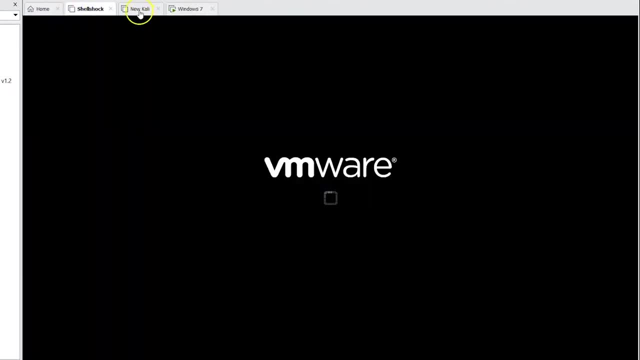 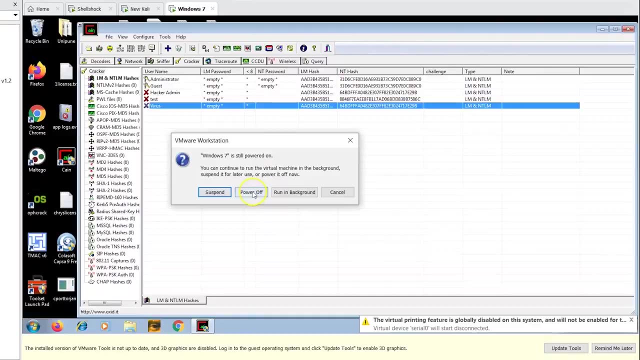 i'm going to do is: this is the linux web server that i have that i'm going to power on. i'm going to use a kali linux machine to hack that device and i'm going to just power off my windows 7 machine. give it a minute till it boots up. now, this is also a demo machine that we have, which. 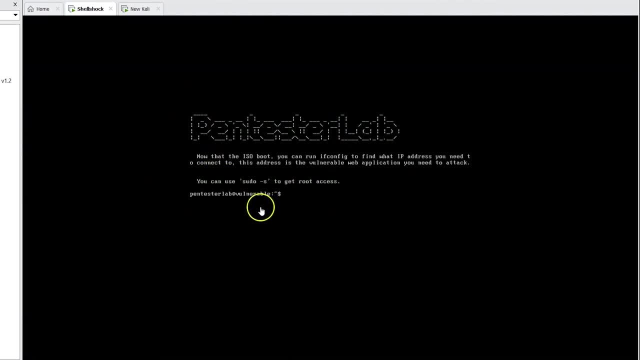 has its own pre-configured vulnerabilities. so here we've got something from the pentesters lab and has a shell shock vulnerability implemented inside. shell shock vulnerability affects linux, mac and unix based operating systems for a particular version of the bash shell. bash is the born again shell, which is 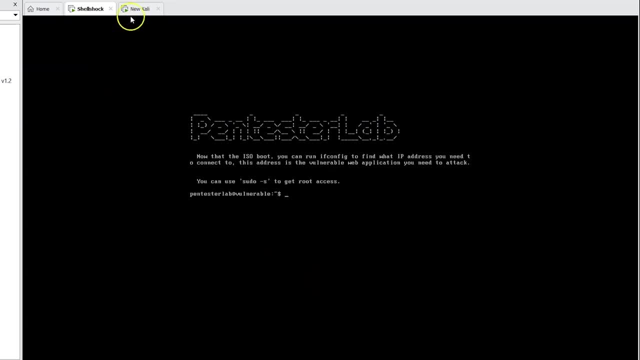 the command line interface in these operating systems. so what we are trying to do here is we are going to use the kali linux machine, try to find out the vulnerability over here and, if it exists, we are going to use metasploit to attack this machine. now, the first and foremost. 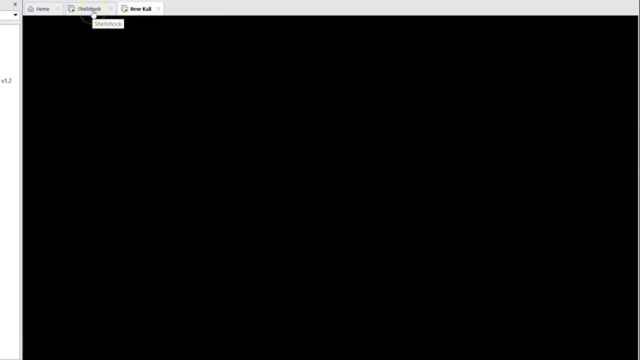 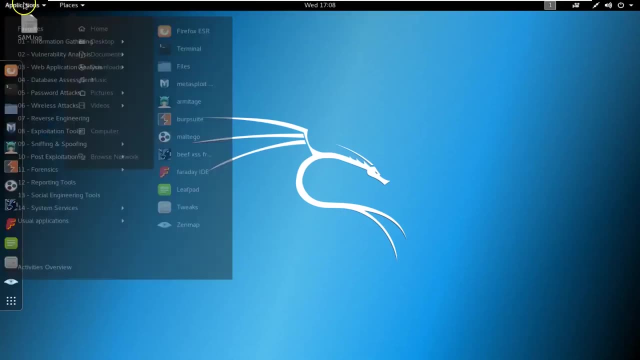 thing is, we want to identify the ip address. we have no idea what the ip address is. we are in the same subnets, so we are assuming that we are able to connect to this machine. so what i'm going to do is i'm going to open up a tool called zenmap. i'm going to open up a command line interface: find out. 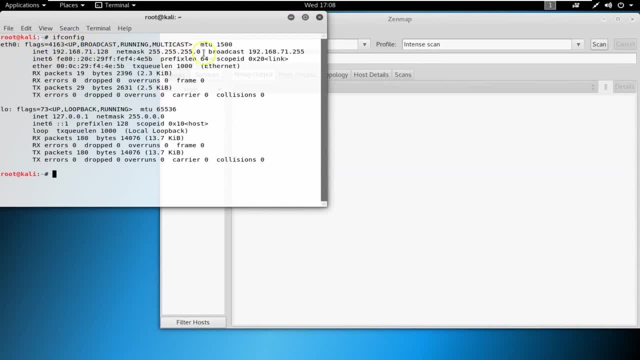 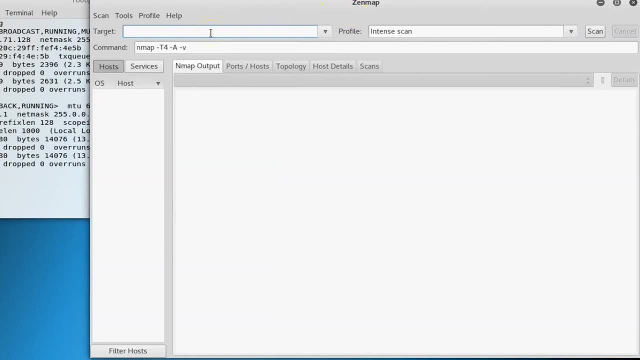 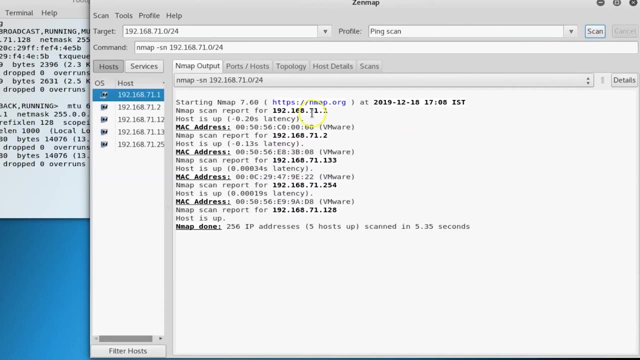 what my ip address is. and my ip address is this, with a subnet mask of 255, 255, 255.0. so i want to see if there are any other machines that are live in the same subnet and we are doing a ping. swipe are live. in a minute we'll get all the ip addresses: 71.1, 2, 133, 254 and 128. we know that. 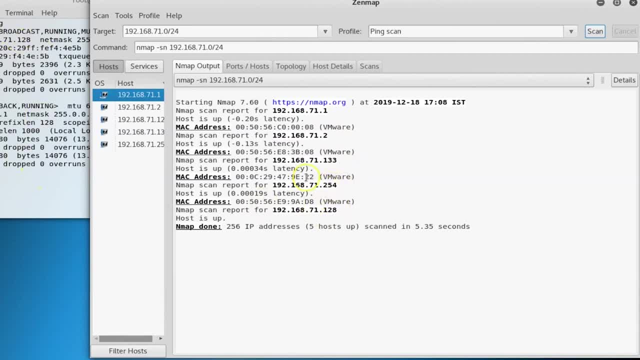 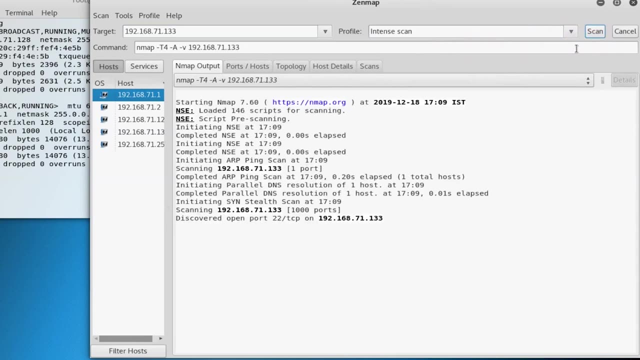 we are 128 at this point in time. uh 254 is the dhcp server. so we are assuming that 133 is the machine that we want to look at and let's then try to see if we can scan that machine 133, and we're going to do an intent scan to find out which ports are open, what services are running over there. 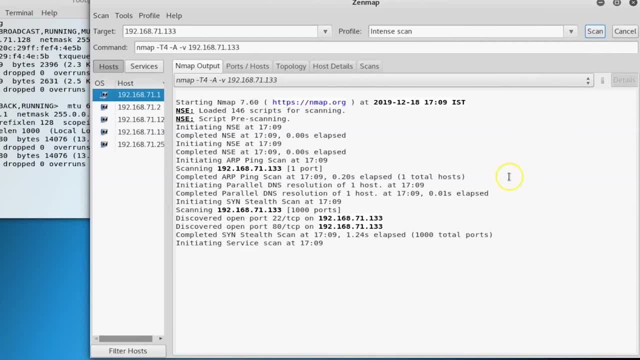 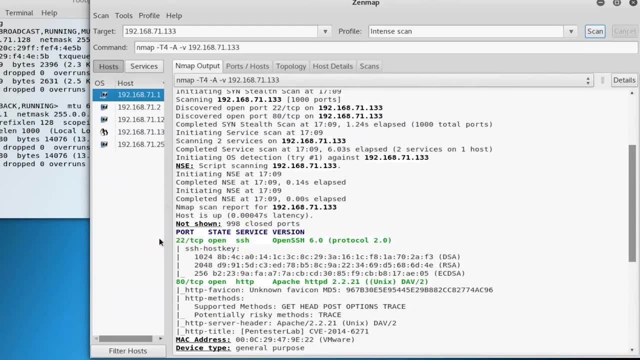 and if it is, whether the pentest machine that we were looking for. you can see of the start, port 22 and port 80, and somewhere here it's going to give us the ports that are open and the details about those ports, and somewhere here it will tell us that this is the pentester lab machine that we 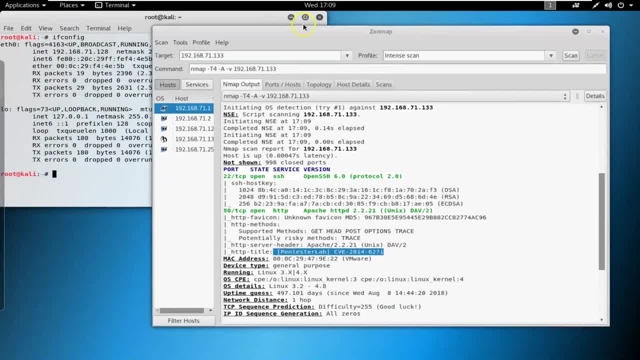 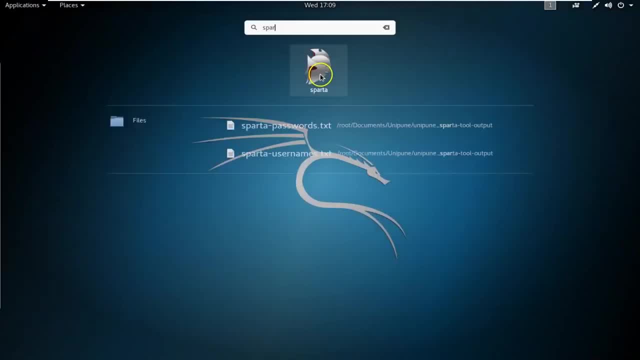 wanted, which is correct. so now we want to do a vulnerability analysis on this. what we are going to do is i'm going to use another gui based tool called sparta, which i can just find out from here. sparta uses two tools in the background. sparta uses two tools in the background. 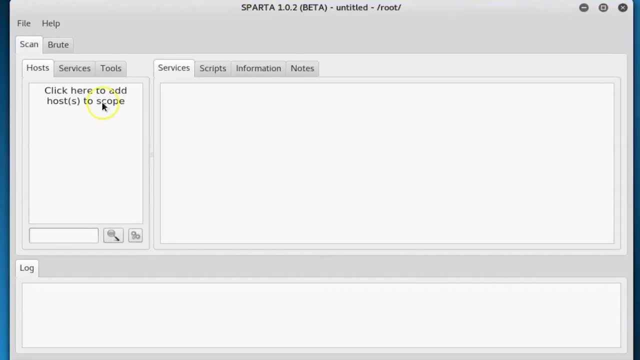 sparta uses two tools in the background: the nmap tool and a tool called nicto, so we're just going to start scanning. 192, 168, 71.133 was the ip address. add to scope and over a period of time you can see all of these will start. 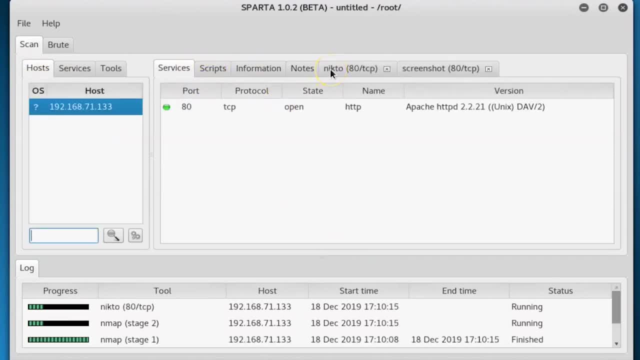 populating with information. there we are. that's the nicto tool coming in, scanning on port 80, which is uh, which means that it's a web server using http. it tells us it's an apache, httpd 2.2.21, and that gives us the 22 port number as well. if we head over to the 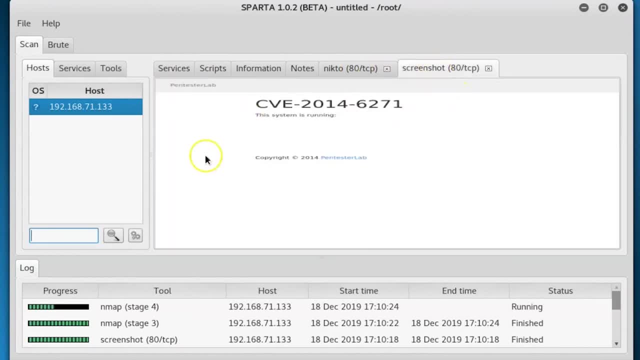 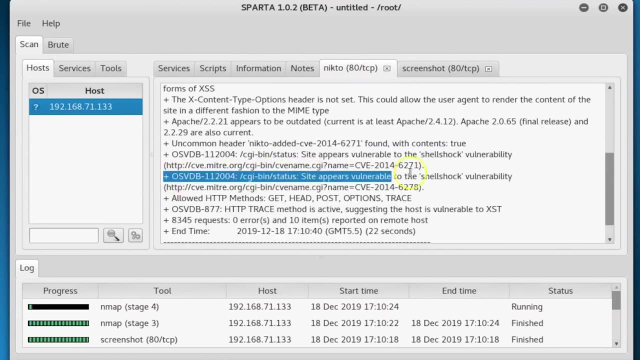 tab of nicto, or let's look at the screenshot first. this is what the website would be looking like, and nicto gives us the options over here. it tells us that there is a vulnerability over here for shell shock and this is the path where the vulnerability is going to exist. so what we're 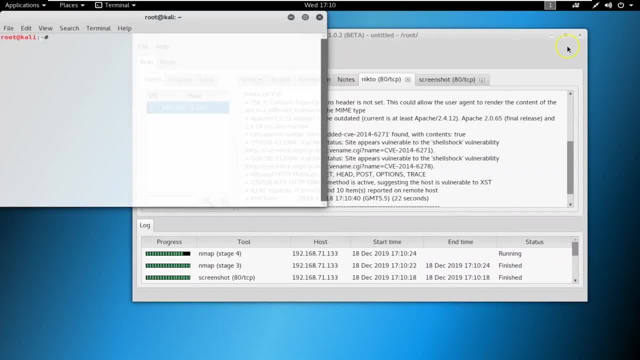 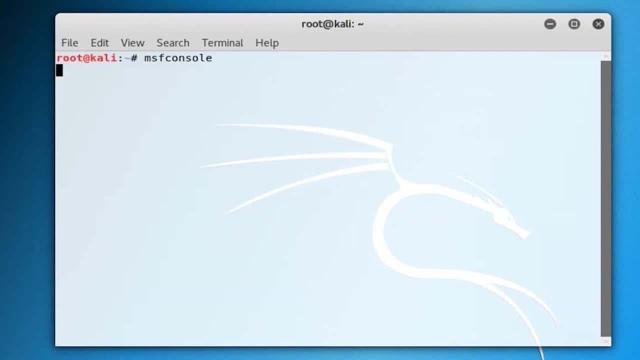 going to do? we go back to the command line? sorry, we open up a new one, minimize all these other windows and we are going to open up metasploit. metasploit is a penetration testing tool that is used by most hackers and ethical hackers to test applications and test uh existing applications. 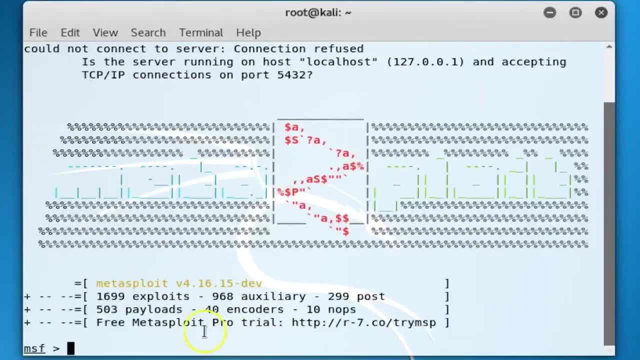 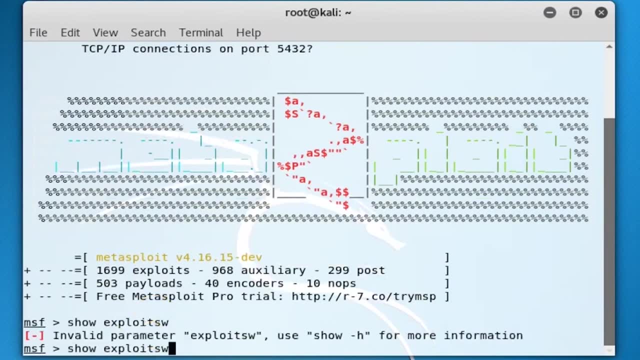 as well as existing exploits and vulnerabilities. so just give it a minute till it starts. you can see there are already around 1700 exploits right here. uh, we're going to see all those exploits with these commands there- we are sorry for the typo- and it will just give us a list of all the exploits. 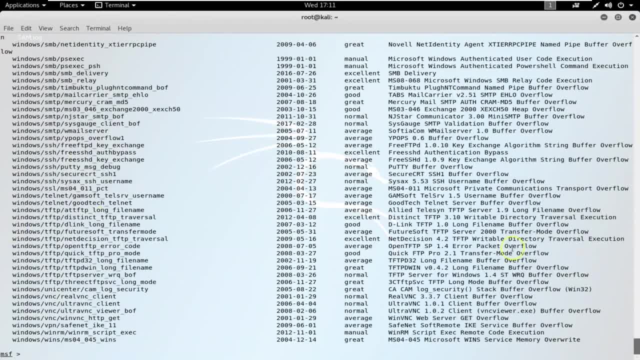 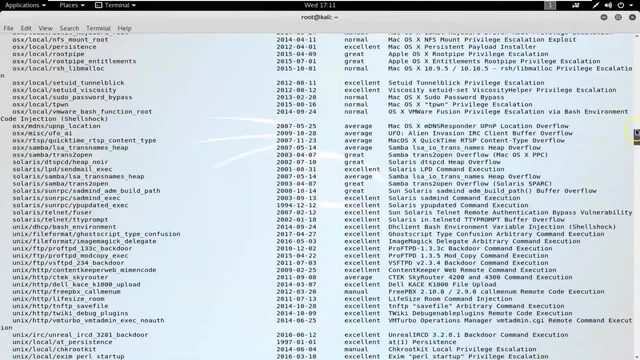 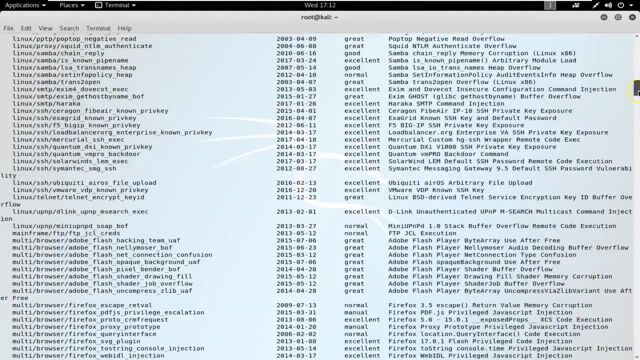 that are stored in metasploit in this version. so all of these are windows based. if we scroll up, we will be looking at other vulnerabilities as well. or exploits, the unique specs exploits, linux, osx multi exploits, and we are looking for a exploit for um multi-based apache or http. let's go up, uh, let's look at. so this is the one that we 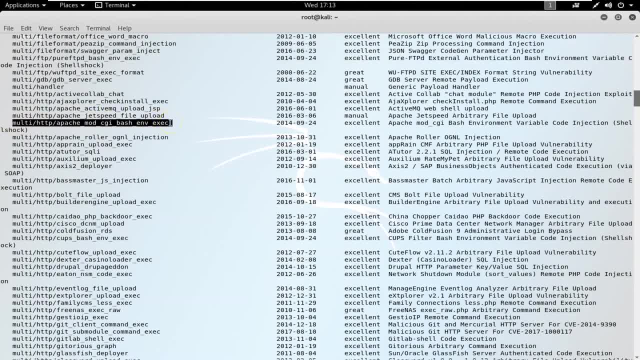 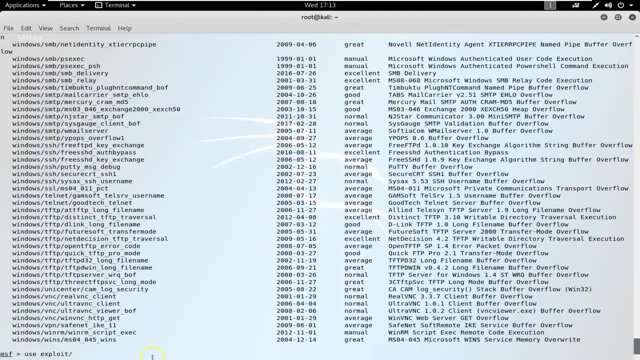 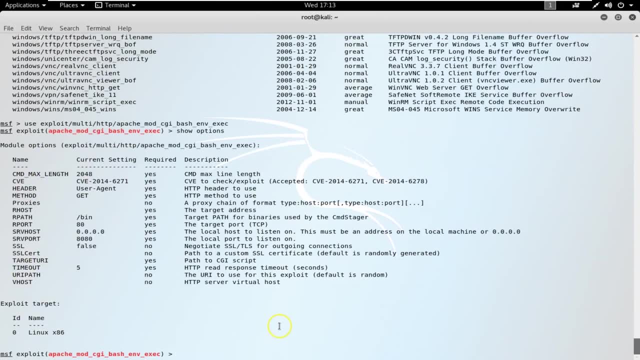 are looking for apache mod, cgi, bash, environmental executable. so what we're going to do is we're just going to copy it. go back to the bottom, say use exploit and paste the one that we wanted. press enter, say show options. so it will ask us to configure this. i'm just going to configure it. 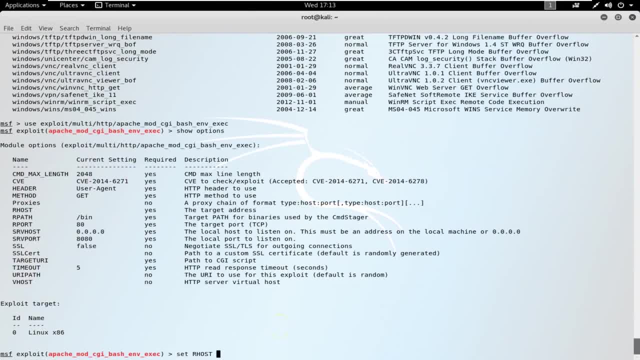 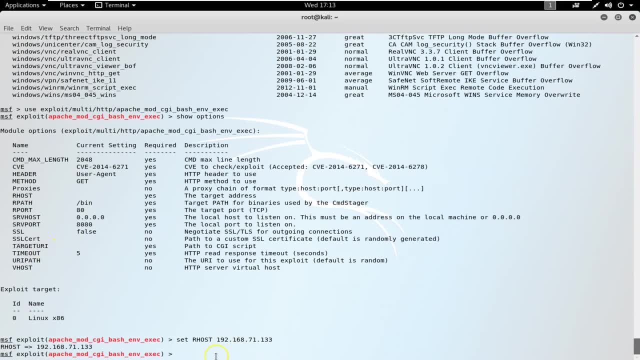 based on the knowledge that we have set our host, which is the one that we are going to use, and then the remote host, the victims machine. so we put in the ip address. it asks us for the target uri. so that's the path that we saw. set target uri to cgi hyphen bin slash status. enter now with the exploit. 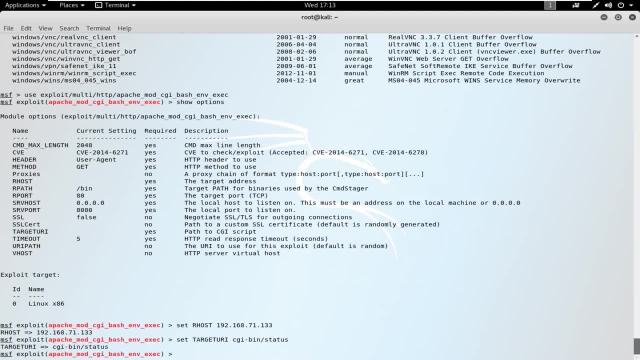 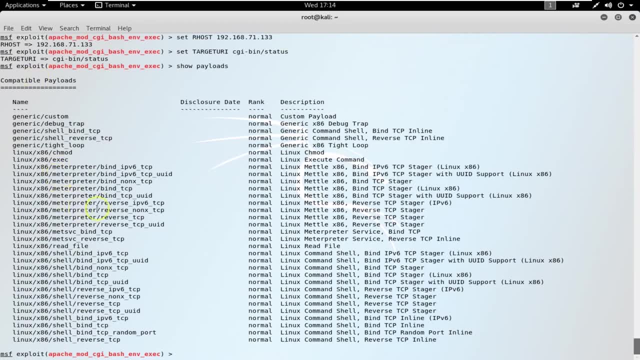 we need to find a payload that is going to give us the output that we want. so we say: show payloads and it will give us a list of all the compatible payloads with this exploit. and we want to create this. so we know it's a linux operating system. we want this payload to be set, so set payload press. 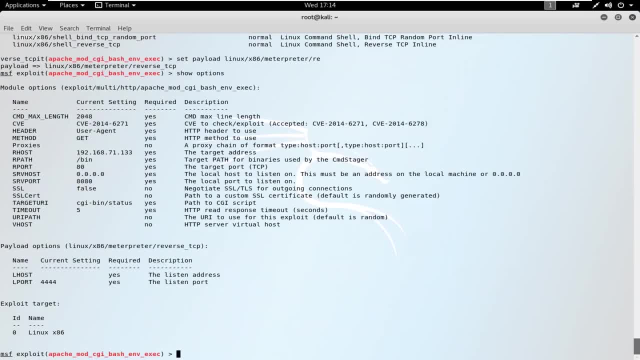 enter. that's the payload coming in. show options now that we have set the payload. this is the options for the exploit, and now we want to set our options for the payloads as well. so we are creating a reverse tcp connection, which means we are remotely executing code at the victim side. 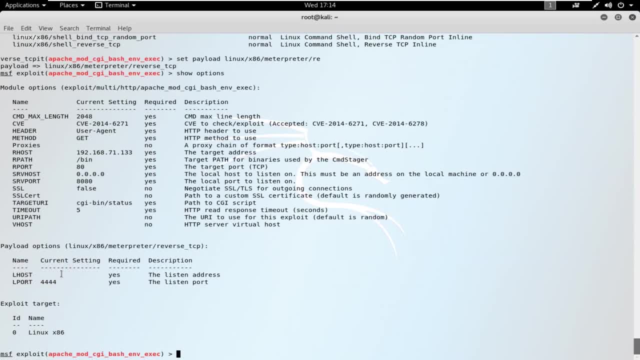 and we are making the victim connect back to our machine, which means we need to set up a listener. so i need to put my ip address over here, set local host or lhost, 192, 168, 71, not 128, which was our ip address. show options again, just to ensure. 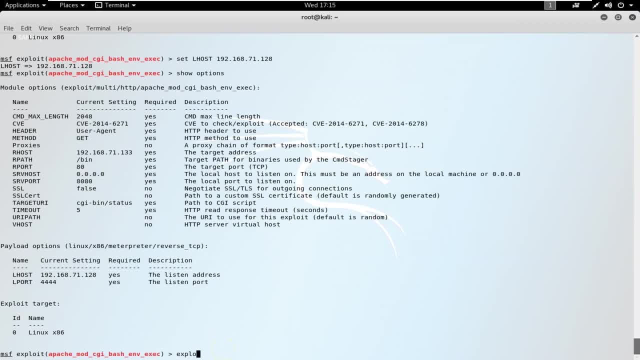 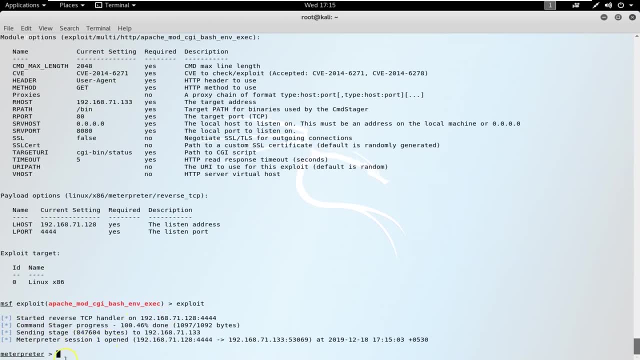 everything is fine, which looks like it is, and we then type in the word exploit so that it will start this attack, i can see that it has created a meter breeder session at the victim site and it has opened up a session. so if i do a pwd now, pwd is a linux command for present working directory. 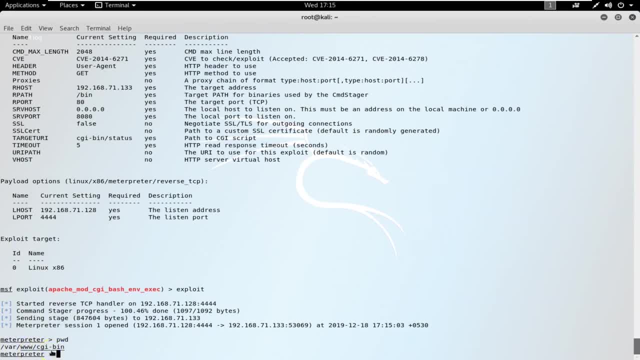 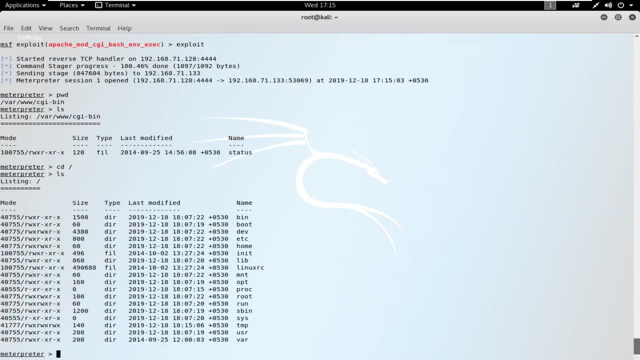 and it will show us that we'll connect it to var. www, cgi, hyphen bin slash status enter and we're going to do a cd backslash. it will list all the files, that's the status file over there. do a cd backslash. it will take us to the root of this machine now. remember we saw the passwords on. 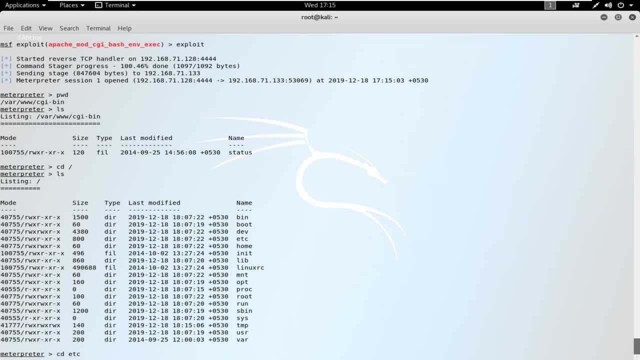 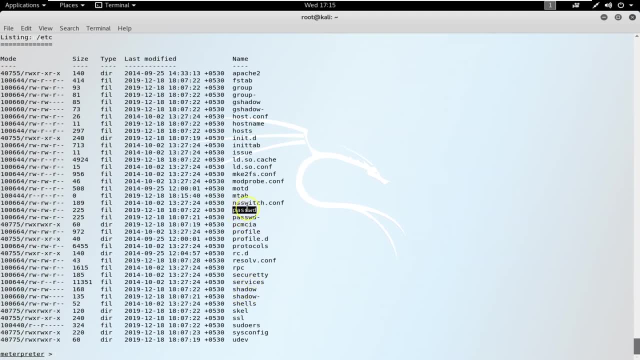 a windows machine. similarly, we can head over to the cd etc. folder ls and you can see these files: psswd and shadow. now, psswd is the file where linux stores its usernames and shadow is the file where passwords are shown. so do a cat command psswd, and you can see these users. 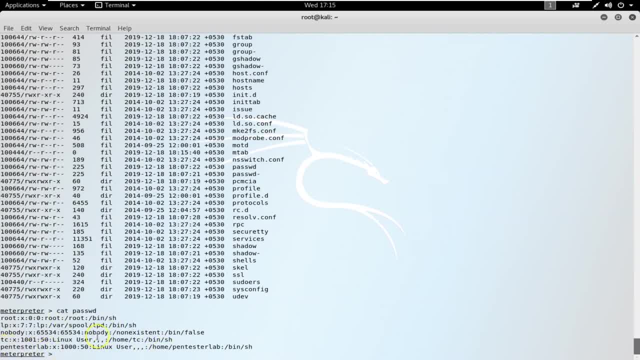 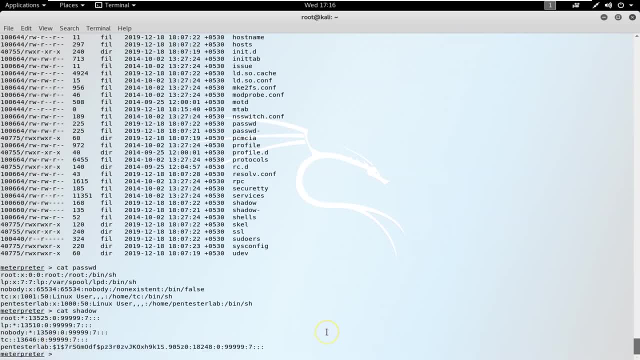 coming up so you can see the last user pentest lab and you can see there are no passwords. so let's do a cat shadow and that's your hash value for the password that we have for the user pentest lab. so these are the different attacks that we need to understand, uh, and we need to create based. 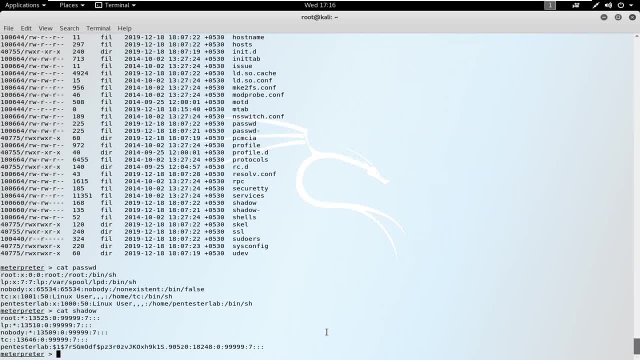 on the vulnerabilities that exist on different machines. so if you just look at windows and linux and how we can exploit them depending on existing vulnerabilities, as a ethical hacker, this is uh what we need to learn in order to be able to exploit these vulnerabilities. so let's take a look at. 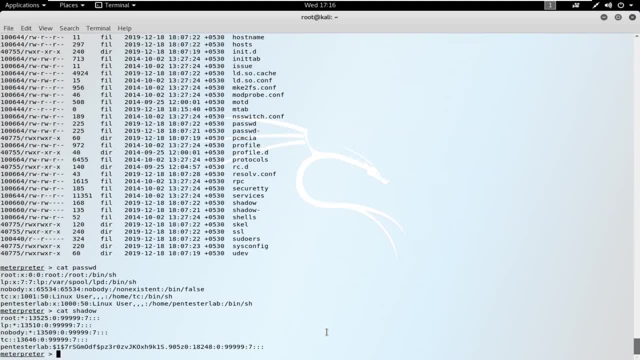 our training and then we need to clear our exams based on this knowledge of how these things work, so that we get certified and then we can position ourselves for the penetration testing jobs. that's it for this demo. i thank you for your patience with me and i'll see you in the next video.